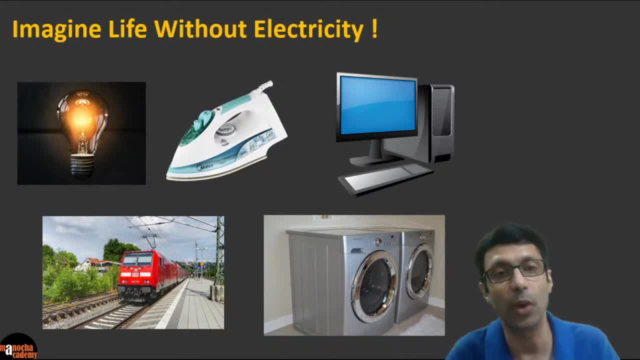 Which was very devastating, And a lot of the electricity in West Bengal and the neighboring state Orissa was cut off And a lot of people's lives were affected during this time. So without electricity, you know, it's a really difficult life these days because everything runs on electricity. 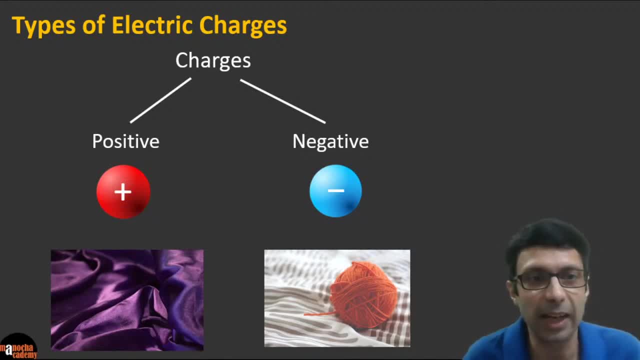 And so, before we start on what exactly is electricity, let's take a look at what are the type of electricity Electric charges. So, guys, what are the type of electric charges? You can divide the charges into positive and negative. So electric charges can be divided into positive and negative charge, right? And how do you get positive charge? You guys must be knowing this, that if you take a glass rod, right. So let's say, I have a glass rod here. 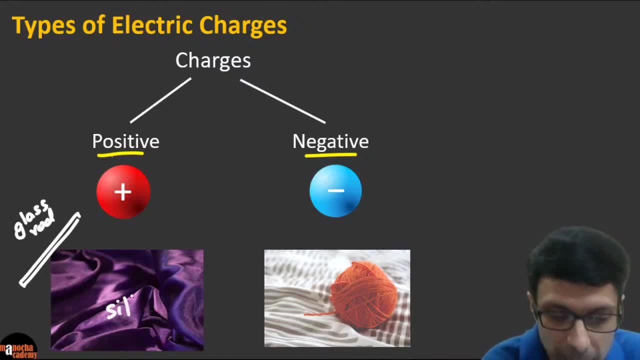 Okay. and if it's rubbed on a silk cloth, You know the glass rod is going to get positively charged, right Guys? the glass rod will get a positive charge. And if you take an ebonite rod, Okay. so if we have an ebonite rod, 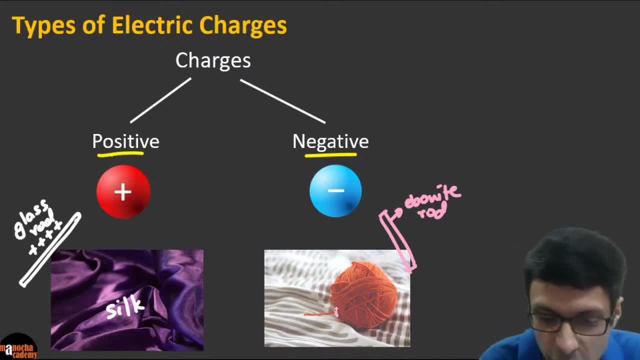 So if you take an ebonite rod and you rub it on wool, So, guys, what is going to be the charge on the ebonite rod? And some of you are asking my name. Okay, My name is Sandeep Manocha, And so do check out our website and our channel website is ManochaAcademycom and our channel is Manocha Academy. Okay, So right And thanks, guys, And do share it out with your friends And guys. if you haven't hit the like button, please hit the like button right now. 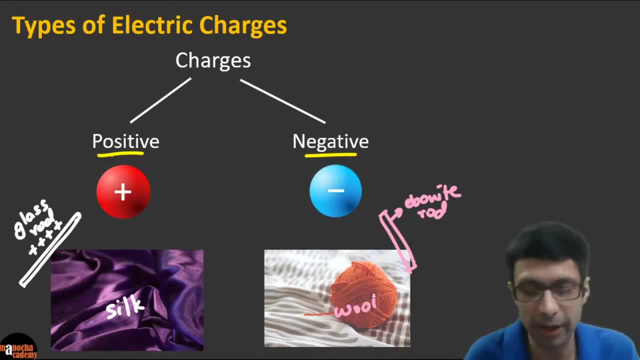 So, come on, I want all of you to try. So when an ebonite rod is rubbed on wool, very good, It gets a negative charge. Okay, so charges can be classified. That's positive and negative, And these have been decided by the scientists. Okay, so some scientists? ah, so the convention has been. 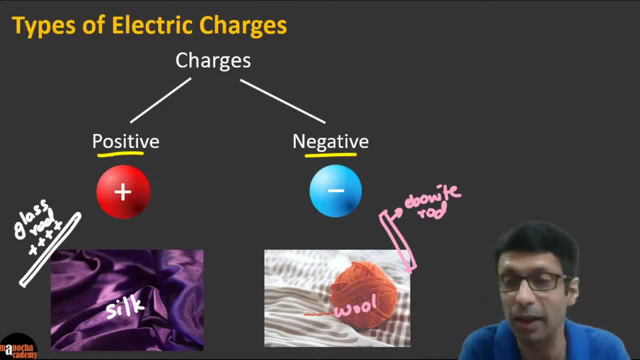 decided by the scientists Right. This team of scientists said: Okay, when glass rod is rubbed on silk, we'll call it positively charged. So this type of charge will be known as positive right. This example: factors of the Kikayi. 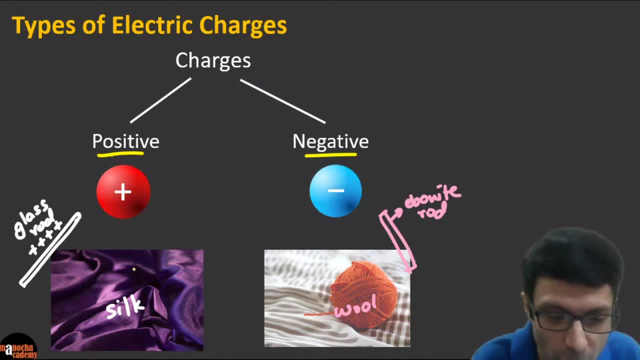 So this type of charge will be known as positive. right This example. and when the ebonite rod is rubbed on wool, the ebonite rod gets a negative charge and the wool, of course, gets a opposite charge. Right, The positive charge. Same way with the glass rod: gets a positive. 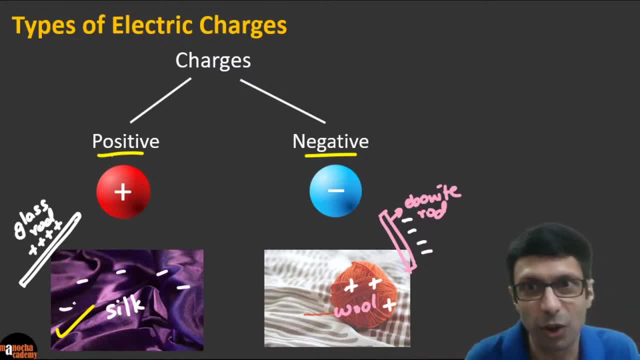 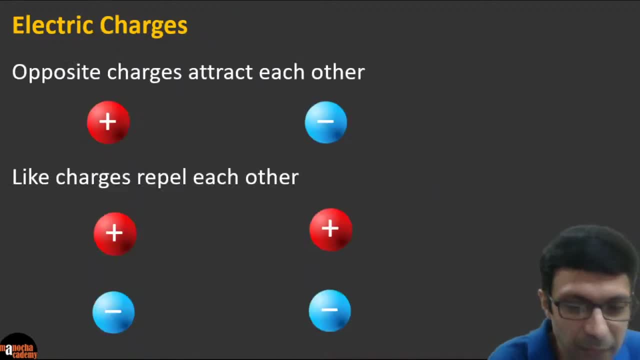 The silk cloth gets a negative charge. OK, clear guys. So these are the types of charges, positive and negative, And all of you must be knowing right that opposite charges attract each other, Like you know about the North Pole and South Pole, Right. 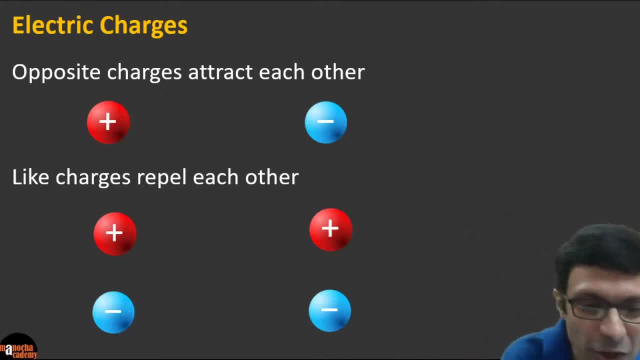 So North Pole and South Pole of a magnet, you know they attract each other. So you know that opposite charges, a positive charge attracts a negative charge, with a force, Right And light charges. Right, Light charges mean similar charges. 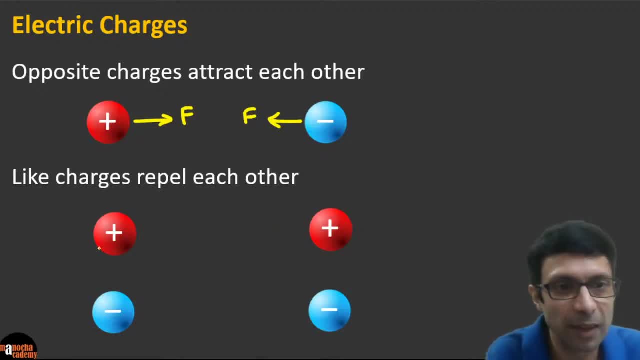 So if you have two positively charged bodies, what will happen, guys? They will be repelling each other, Right, guys? So two positively charged will be repelling each other. And what about two negatively charged bodies? They will also repel each other with a force. 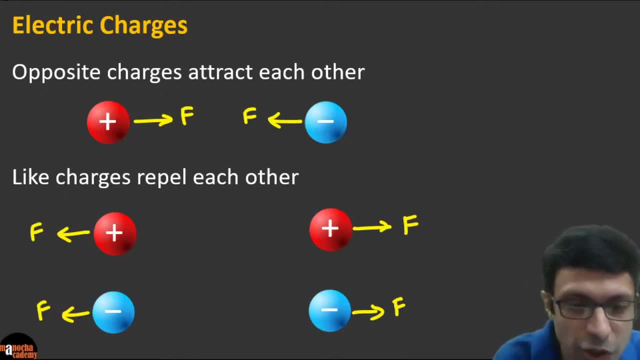 OK, So, as you can see from the picture here, so light charges- they repel and opposite charges they attract each other, Right? So is that simple, Right? So these are the basics of charges. I think all of you know about these simple concepts. 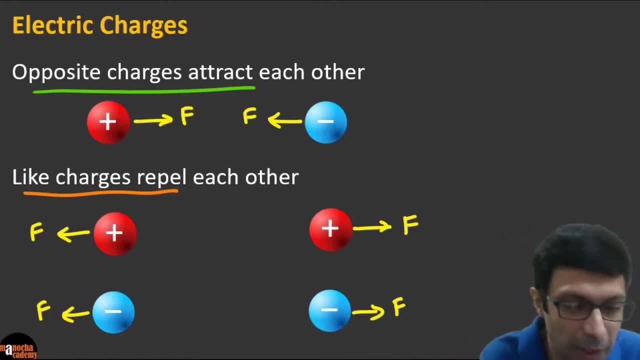 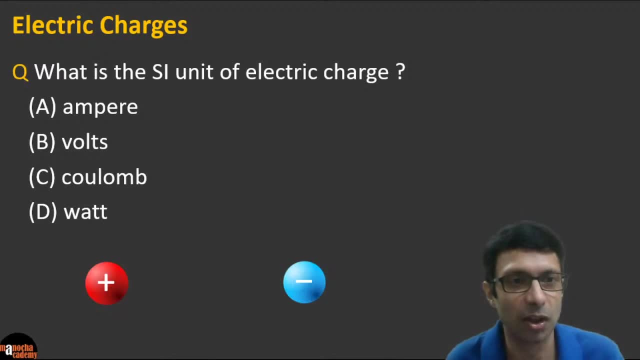 Or if you don't know, don't worry, We are going to discuss a lot of things about electricity today. OK, it's going to be an electrifying class, And what is the SI unit of charge? So, guys, what do you think? What is the SI unit of charge? 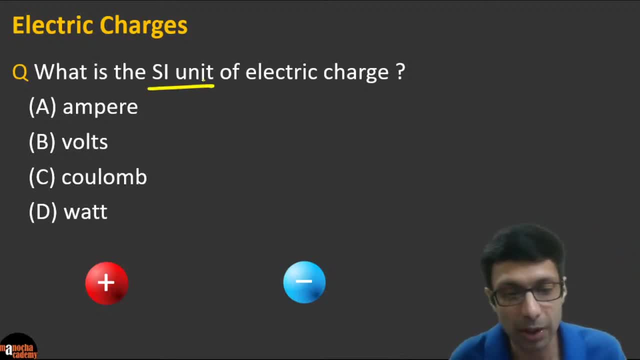 Electric charge. Is it ampere, Is it volts, Is it coulomb Or is it watt? What do you guys think? And I want all of you to try in the chat here I'm taking a look at the chat, So I want all of you to try. 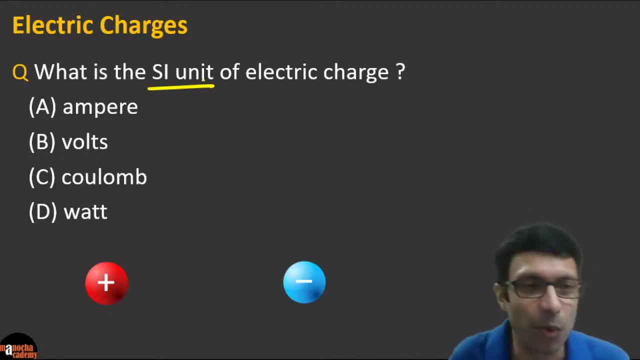 And it doesn't matter if your answer is right or wrong. OK, this is not a test. We want everybody to get to attempt the questions. OK, OK, Excellent. I see Vinay Manu, They're saying coulomb. OK, Himanshu says coulomb, Excellent, guys. 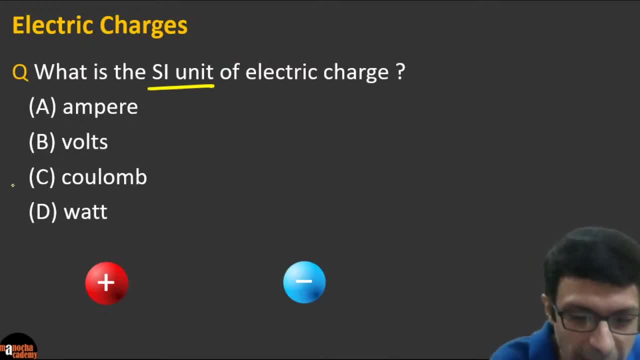 Please remember the SI unit of electric charge. The right answer is coulomb, And we need to remember this because it's not that we use coulomb in our everyday lives, Right? It's not often used. OK, so coulomb is the SI unit of electric charge. 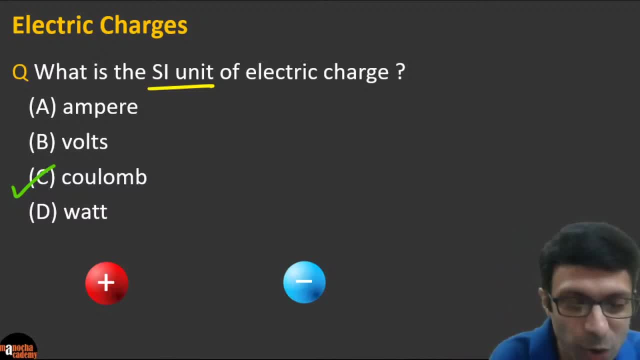 Clear guys And the spelling. Please note the spelling. OK, So it's C-O-U-L-O-M-B, So I remember the word. You can say the word as coulomb- Coulomb. OK, So sounds cool. 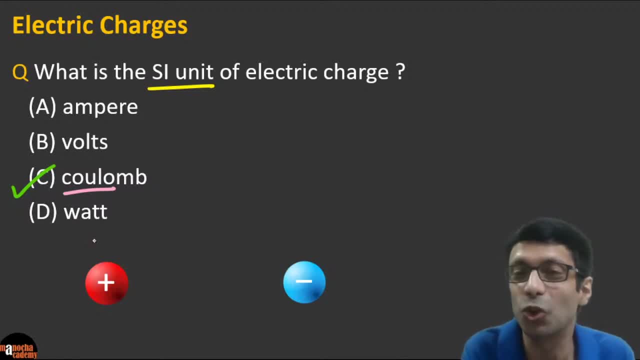 Right, guys, But it's not C-O-O-L as cool, It's coulomb. So please note the spelling. And what is the symbol for coulomb? It's the. it's denoted with a capital C. OK, so coulomb, Right. 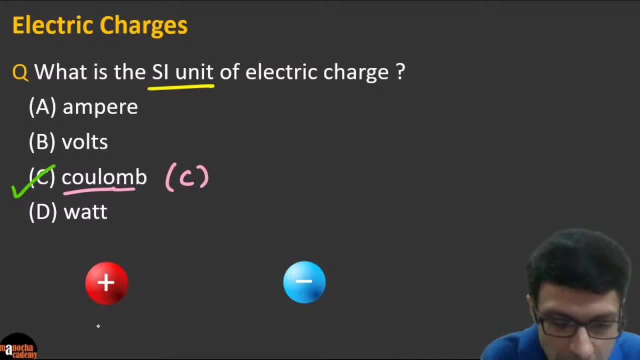 So, for example, we say this body has a charge of: if it's a positively charged body, we can say this has a charge of plus five coulomb capital C. Right, Let's say this is a negatively charged body. It has a charge of minus two coulomb. 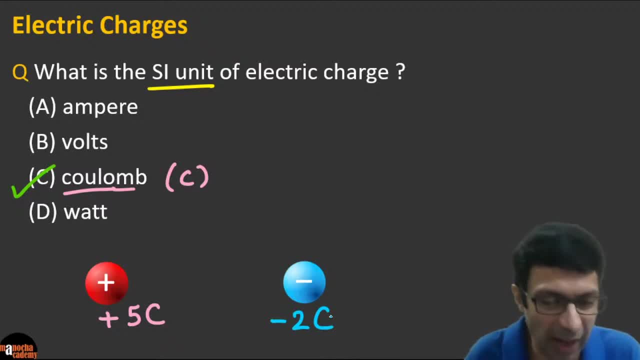 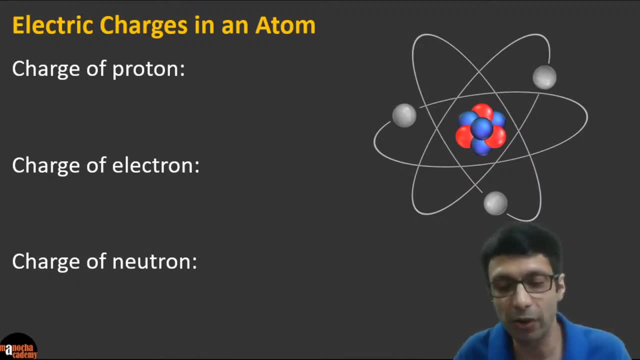 OK, Where capital C stands for coulomb. Excellent guys, Very good, And you must be knowing this Right, That a lot of you have studied in chemistry, Right On physics, that an atom is made up of subatomic particles, Right. 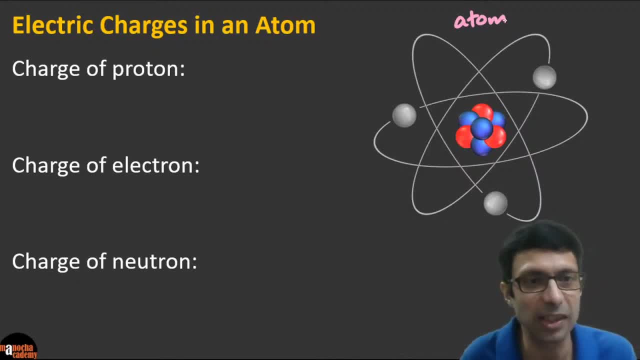 You've heard of these subatomic particles- protons, electrons and neutrons. OK, So, guys, can you tell me what is the charge of one proton? So let's start with the proton first. What is the charge of a proton? 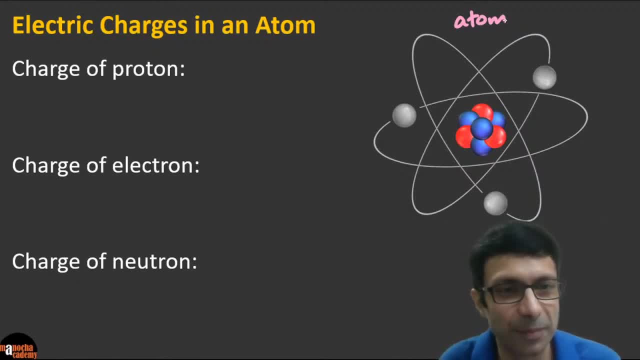 Come on, I want all of you to try. Come on, guys. Excellent, Excellent. I see Aditya Prakash Very good. A lot of you, Yes, A proton guys. So let's look in this picture here. 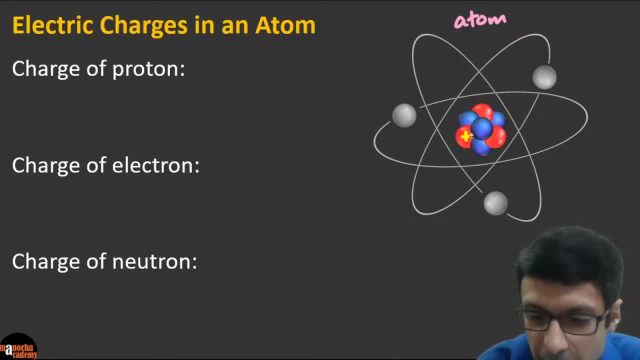 You know, proton are these positively charged particles. So these red ones are the protons here, OK, And the gray ones are the electrons, the negatively charged particles. And you know what is the charge of a neutron Neutron is has no charge, Right? 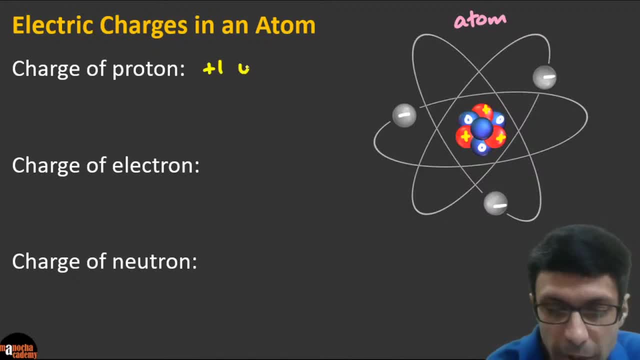 Roughly speaking, we can write: charge of a proton is plus one unit Right, Charge of an electron is minus one unit and charge of a neutron is zero. Basically we say it's neutral. OK, And this unit is because it's a very small amount of charge. 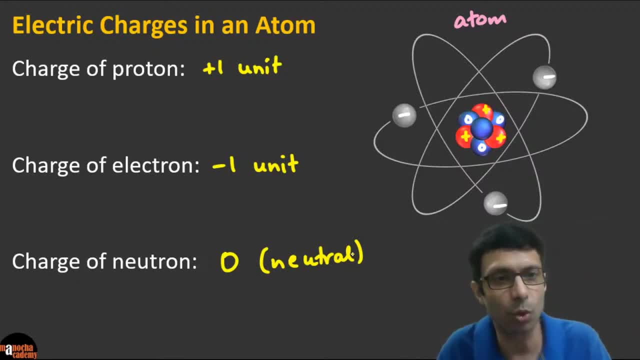 So we just say plus one unit. But if you want to write it in SI units, it's a very tiny charge. And remember we said what is the SI unit of charge? We just talked about it: Coulomb. So how much is the charge of a proton in one coulomb? 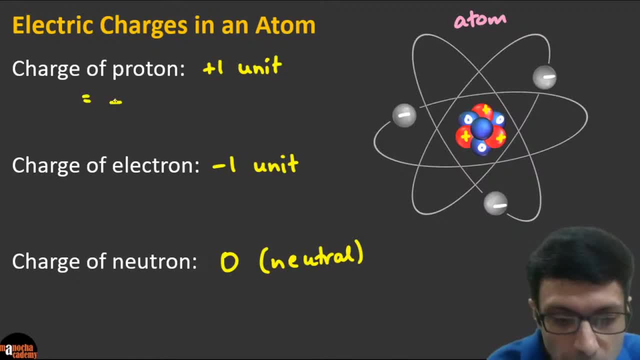 In a coulombs. you need to remember that. So that's going to be equal to plus one point six into ten, to the power minus 19 coulombs. OK guys, So plus one point six into ten to the power minus 19.. 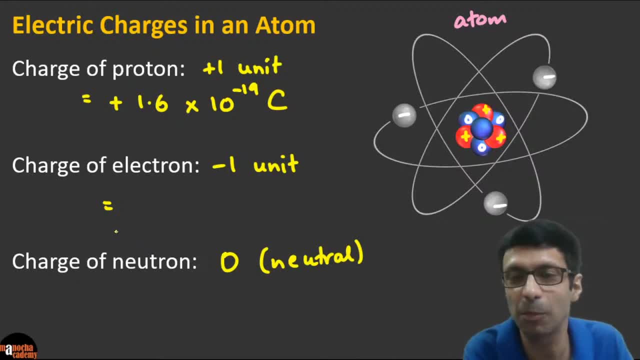 Excellent, Excellent. And electron is exactly same as the proton, except with the negative side. OK, So it's going to be minus one point six into ten to the power, minus 19 coulomb. OK, And what is the charge of a neutron? 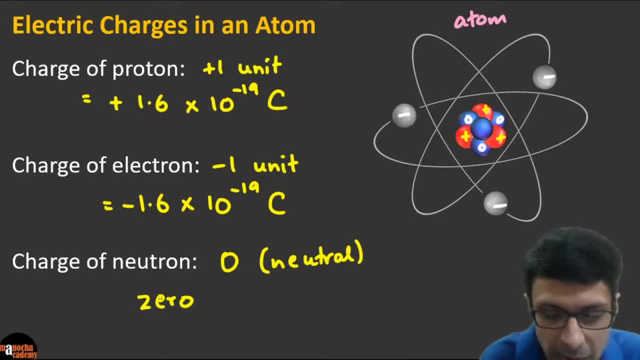 Neutron has no charge, It's just zero Right. So we can say it's zero coulombs, Clear guys, Excellent. So please remember this very important value: One point six into ten to the power minus 19.. Right Minus 19.. 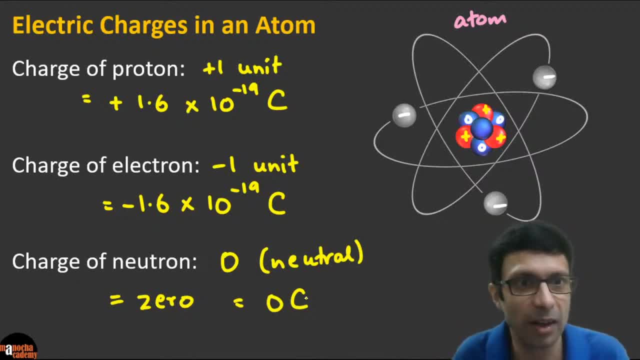 It's a very, very small amount of charge. OK, Very good, Awesome. And you know that these, the atom is made up of these subatomic particles which are charged particles. Right, Because we are talking about electrons, We are talking about electric charges. 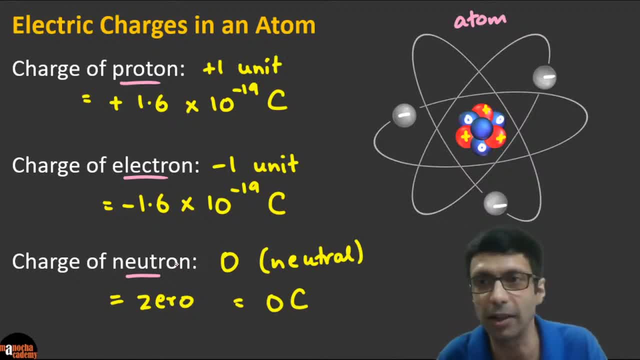 So we have to note that protons, electrons are the charged particles in an atom. And but, guys, what is the charge of the atom? The atom itself has zero charge. It's neutral because the protons and electrons, they cancel each other. 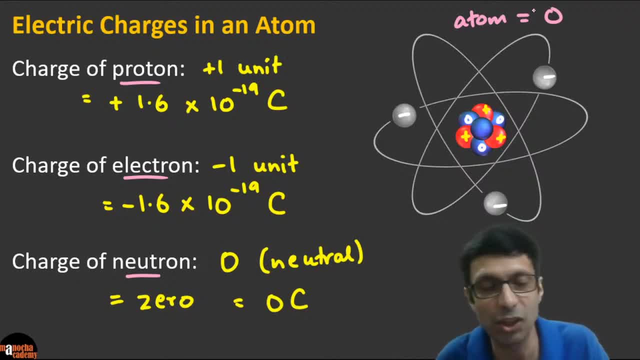 OK, The charge. the charges of a proton and electron will cancel each other. So the atom is neutral, neutrally charged. OK, It has no charge. Excellent, guys And guys. if you haven't hit the like button, please hit the like button. 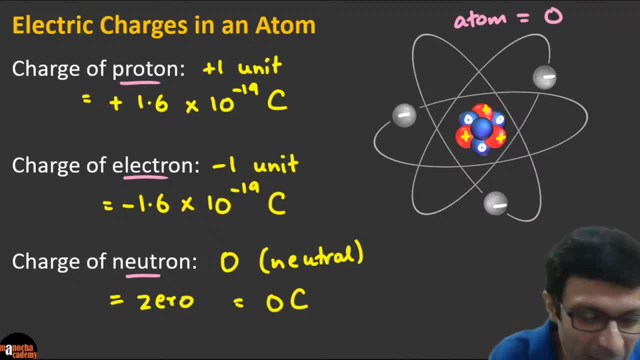 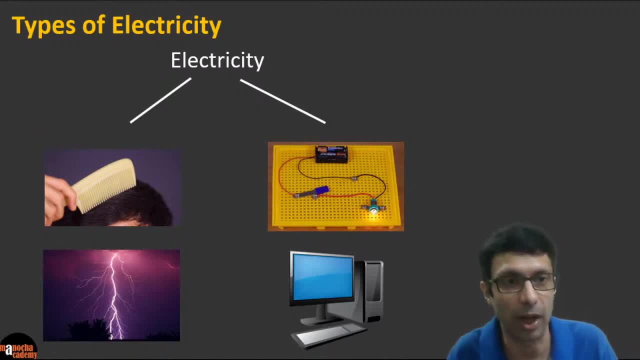 And do share it out with your friends. OK, So let's move on to. So we talked about electric charges. Right, And even electricity can be classified into two types. So let's talk about what are the two types. So you must have heard this famous experiment that if you take a comb, 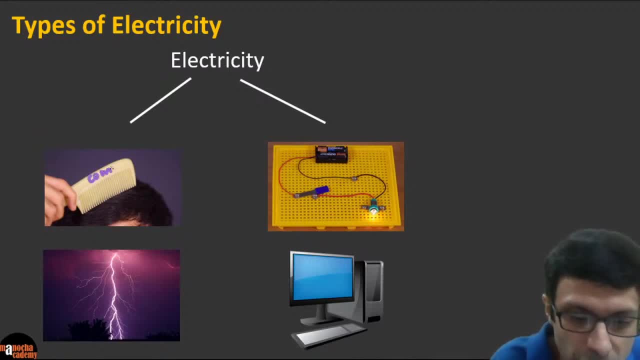 Right, So can you see in this picture? there's a comb here. So if you take this comb and you rub it on dry hair, Right, So you can see I'm taking the plastic comb here and rubbing it on my hair, Right? 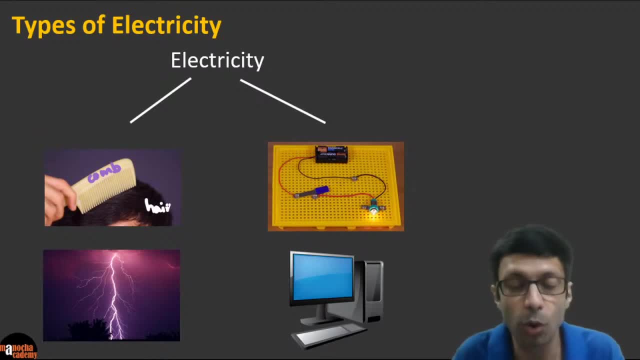 And it has to be dry hair, not wet. OK, Then you know what happens, Do you know? Very good guys? Excellent, Some of you are writing that. So you know that the comb will develop a charge. The comb actually becomes negatively charged. 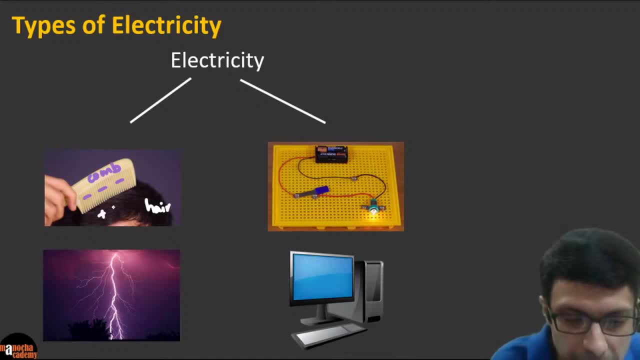 OK, And the hair becomes positively charged. Now, why is that? Because electrons, very important concept guys- because electrons move from the hair to the comb. OK, So there is a transfer of electrons. OK, So there is a transfer of electrons. 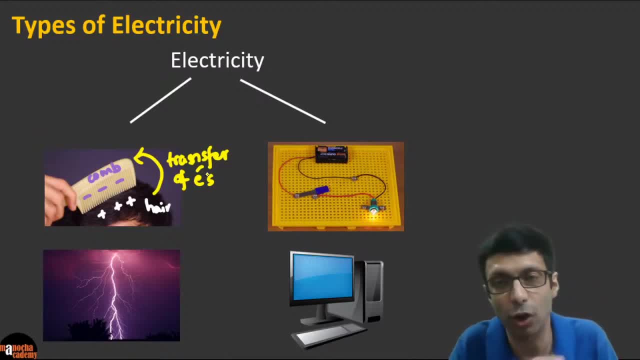 So just like the glass rod gets positively charged because the electrons get transferred from the glass rod to the silk cloth, similar, and the ebonite wool, So similarly here, guys, the electrons will get transferred from the hair to the comb. And excellent. I see Kirit Ayush very good. 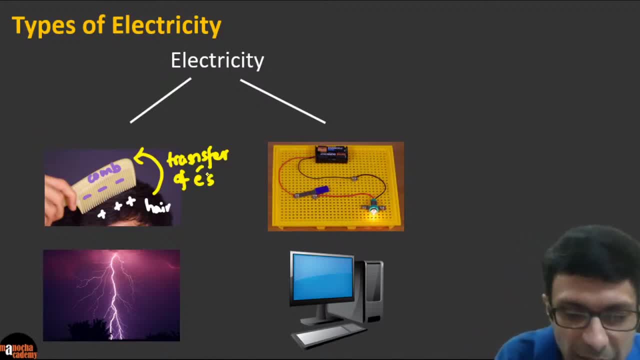 Srinivas Abhishek. they're saying this type of electricity, superb guys, is known as tachycardia. They're saying this type of electricity, superb guys, is known as tachycardia. OK, Why the word static? 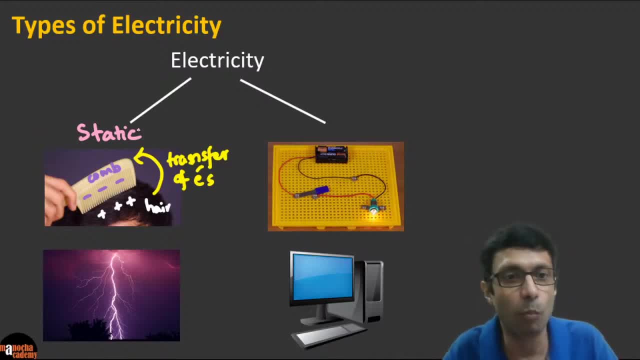 Because there is just a transfer, OK, There is no motion or movement. There is a. there is a movement of charge, but no continuous movement, just a single time transfer, And this is called static electricity. OK, So this is an example of static electricity. 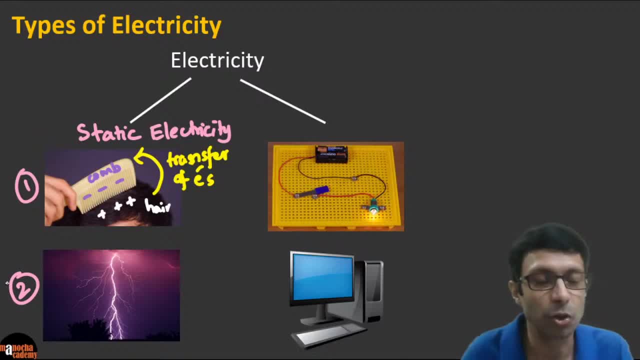 This is one example And, guys, you know the lightning Right. So, Calcutta, we had a lot of lightning, thunder. We are having a lot of bad weather this week and next week also is predicted, So a lot of lightning is happening and lightning is also due to static electricity. 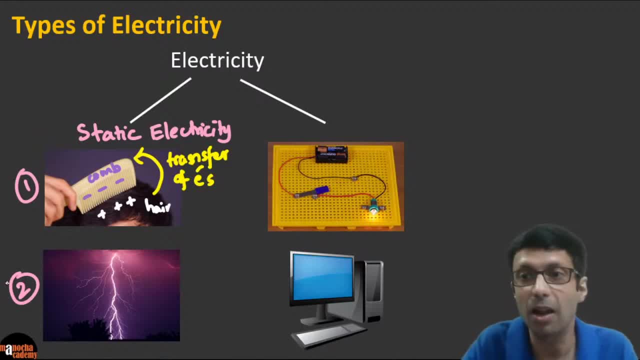 OK, So these are examples of static electricity. Now there's another type of electricity which we are using all the time. Right, That runs our computers, lights, fans. So what is that type of electricity? So come on, guys, Very good. 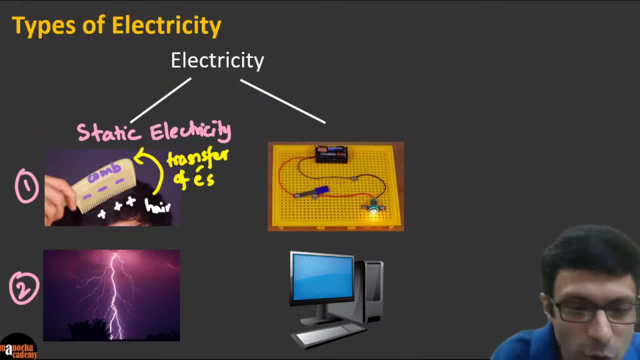 Very good, I see Sonal has the right answer. Excellent, That's called current electricity, Right? So one is static electricity And you can also have static electricity, So we have current electricity, Right, guys? So current electricity is an example. 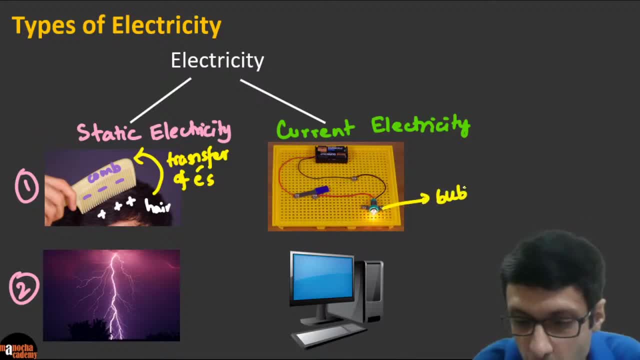 Can you see this bulb is glowing in the picture here? So the bulb glows Right And that is an example of current electricity, because current is flowing in the wires. So we have current flowing in the wires, or we should say charges are moving. 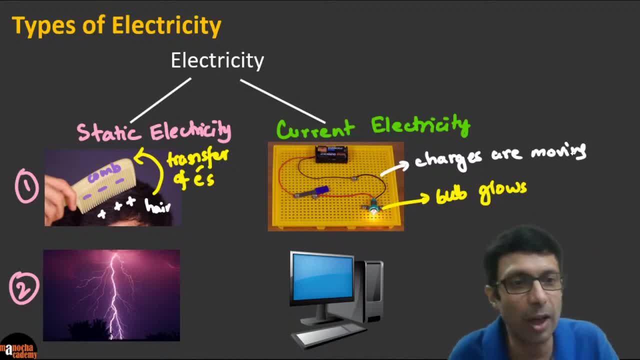 OK, So the important thing is that there are some charge Particles, because you know, electricity is about charges, Right? So there is charge moving continuously in the wire. OK, So there is continuously some motion of charge happening in these wires which is causing the bulb to glow. 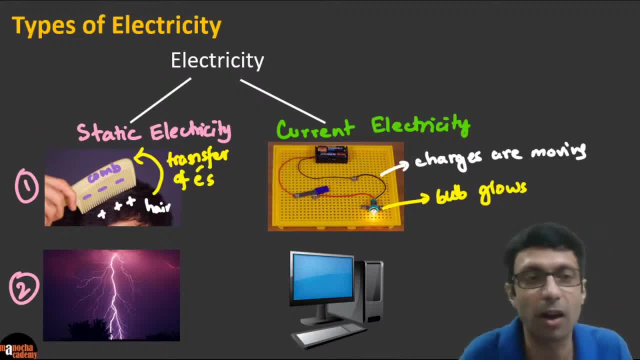 And same with your computer, Right? So these are all running on current electricity, Right, You've heard the word current electric current. So this falls in this category. And what is the important thing? Continuous motion, Continuous movement of charges. OK, So, continuous movement of charges, and that is current electricity. 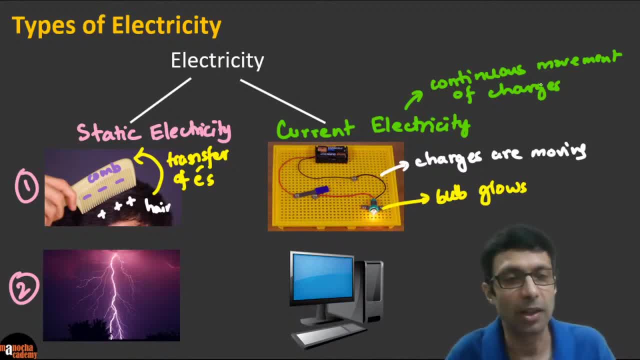 Excellent, Right. So some of you asking which class this is for, This is for class nine, ten, Some of you who are in seven, eight. Also, it will be helpful for you, Right? So anybody who wants to learn the basics of electricity and get it crystal clear, this class is for you then. 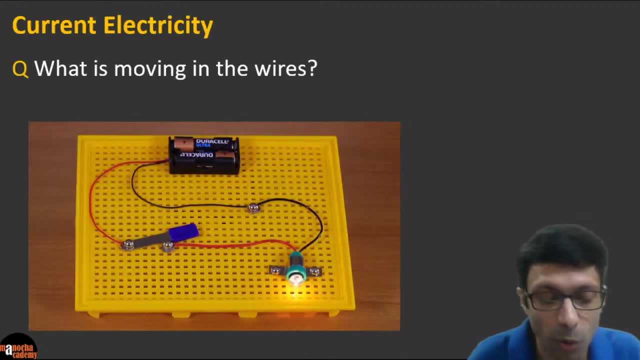 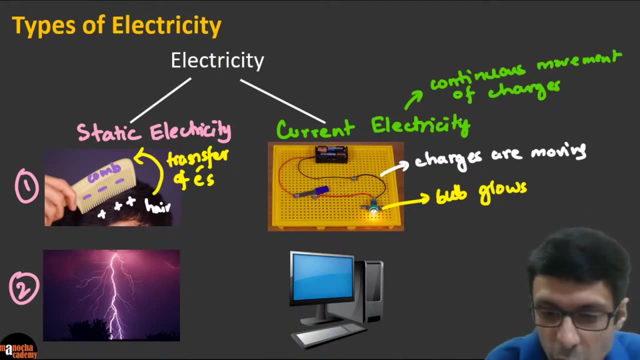 All right, So this part is clear. Let's continue, Right So? and our focus in this class is actually going to be on current electricity, Right So? let me mark that here. So this will be the focus of our class: It's going to be on current electricity. 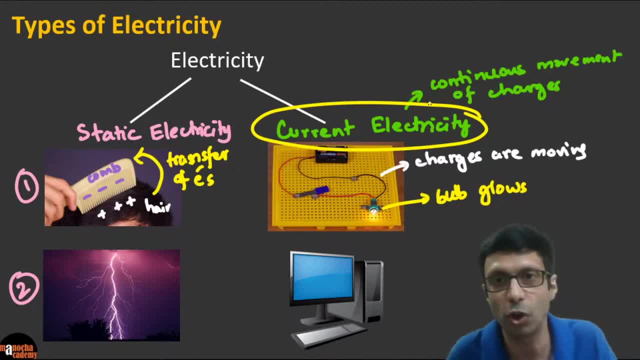 Right, We won't be focused too much on static electricity. So we talked about that transfer of charge, the, the glass rod and silk cloth, the ebonite rod and wool and the common hair example. They are the transfer of electrons. OK, But this continuous motion which causes current to flow through is what we're going to talk about. 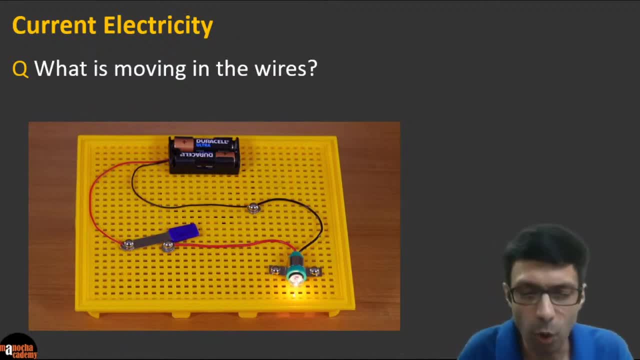 So let's look at current electricity Right. So we said what is moving in this. So can you see that this set up, Can you see the bulb is glowing here? So clearly current is flowing Right, The bulb tells us. because the bulb glows. 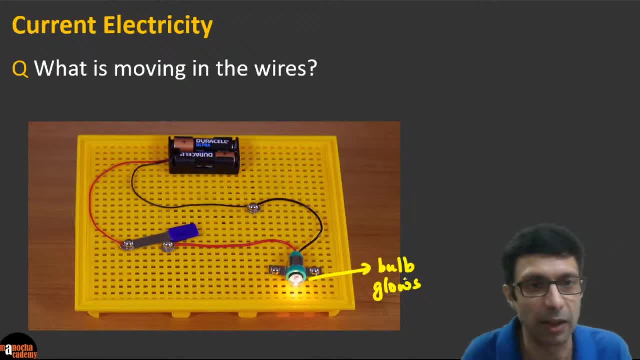 So definitely there is current electricity present in this circuit, Right So in this set up. and what is moving in the wires? Right? So we know that guys, charges are moving Right, But can you tell me exactly what charges are moving? So, is it protons, electrons? 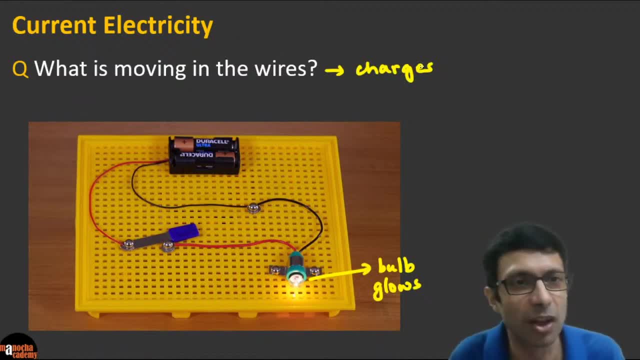 It can't be neutrons, Right, Because neutrons are don't have any charge. So what do you guys think? Excellent, Excellent guys. I see science is life, Right. Rokia Shreyash: very good, You guys have the right answer. 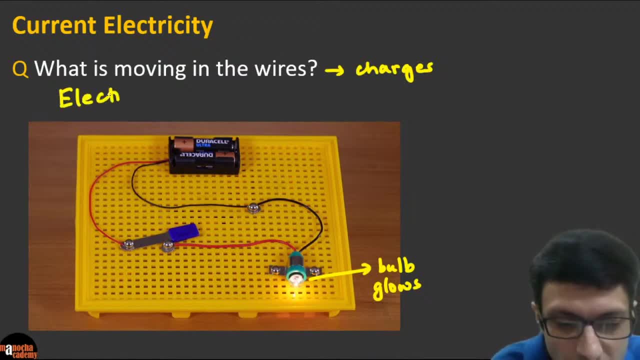 Absolutely correct. What is moving in the wires, guys? Electrons, electrons, the tiny charged particles, Right And as we learned, electrons are negatively charged particles, So negatively charged particles, And it is These negatively charged particles that are moving in the wire here, guys. 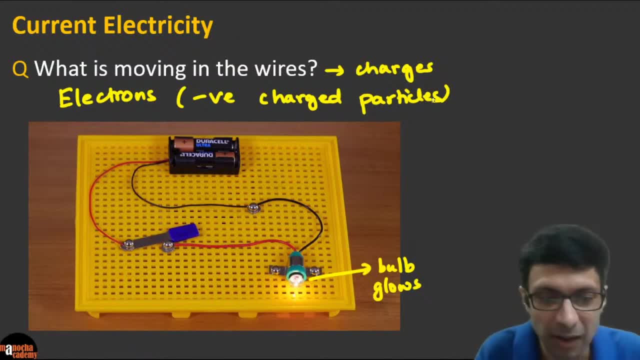 So the negatively charged particles moving in the wire is causing current electricity. OK, so they are flowing in these wires. So let's write that down, guys. So it's the electrons that are electrons which we symbolize with this e-symbol. Electrons are flowing, or we say moving in the wires, and that is causing the bulb to blow. 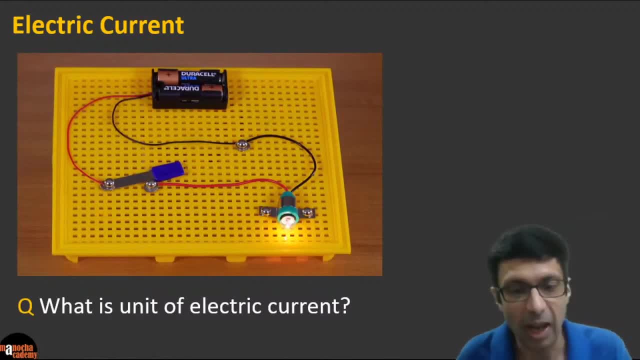 Superb. Absolutely right, You guys rock, OK. And so we can talk about this movement of electric charges Right. That is known as electric current Right. So what is electric current? We can define it as the flow Right, The flow of electric charges. 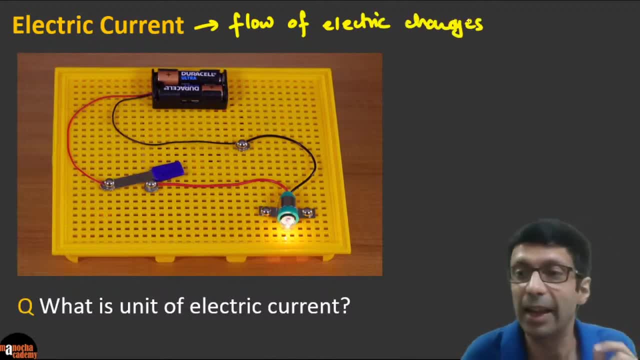 Right. And here we know the electric charge that is moving is electrons. It could be protons also in some other situation, But usually you know, the electrons move Right Because the electrons are the light particles, Right, And they are not in the nucleus of the atom. 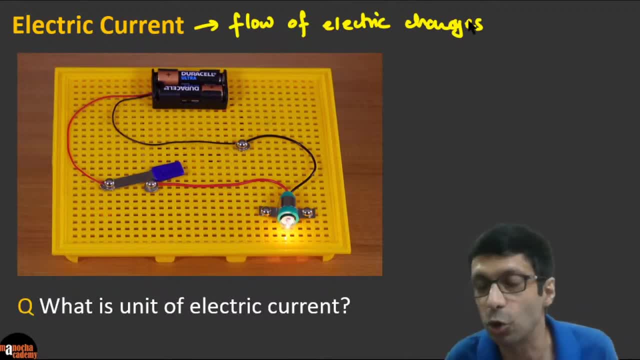 The protons are tightly bound in the nucleus of the atom, And so the protons cannot move. Well, the electrons can easily move, Clear guys. So the electric current is due to the flow of is defined as the flow of electric charges. 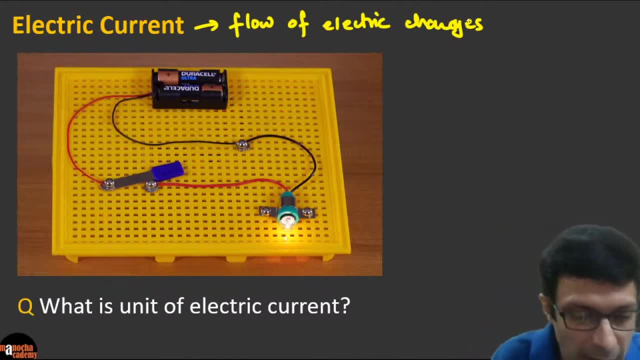 OK, excellent. And how do we define electric current Right? So electric current is also. how do we give it a numerical value? It is the rate of flow, So current can be defined as the rate of flow. rate of flow of electric charge. 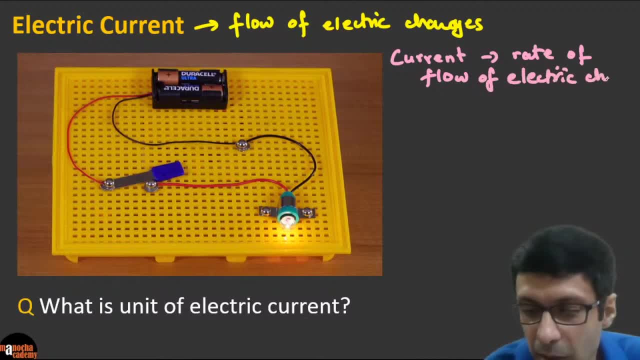 OK, And the current symbol is basically rate of flow of electric charge. The current symbol is I Right? I don't know why they use I for current. I'll have to look that up, But the scientists have. you are using the symbol I for current because C is used for coulombs. 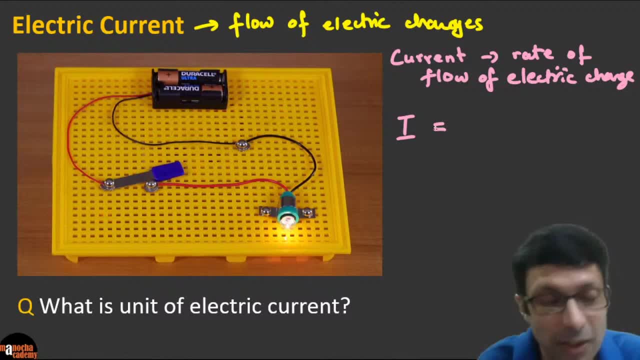 Right, So they can't use C again. Right? So I Right Is equal to, and Q is used for charge guys, So the symbol of charges Q, So let's write that down. So I is equal to Q divided by time. 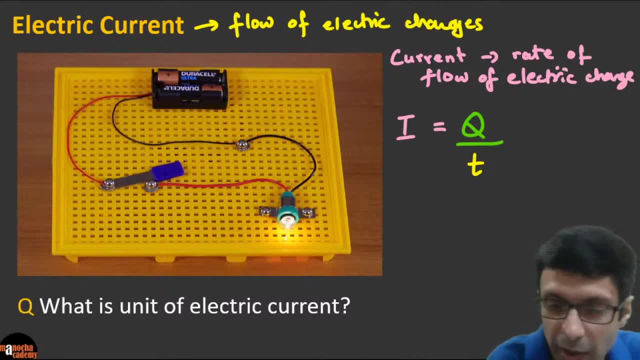 OK, so I is equal to Q divided by time, where Q is basically charge because it's rate of flow of charge And you know, rate means divided by time. So this is basically your formula of current Right guys. So let's say, for example, let's say we have a, we have. 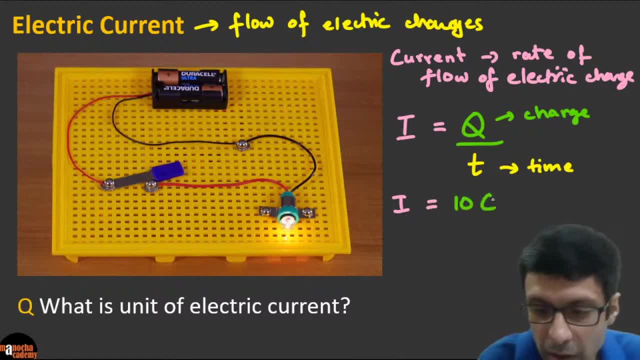 Let's say 10 coulombs of charge. OK, let's say we have 10 coulombs of charge flowing in two seconds. OK, so 10 coulombs of charge flowing in two seconds. So how much current is that? 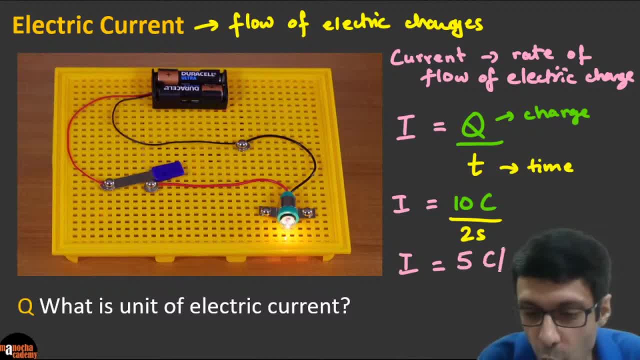 It's going to be 10 by two, So that's going to be five coulombs per second. Right guys, It's going to be five coulombs per second. Now, what is the unit of coulombs here? 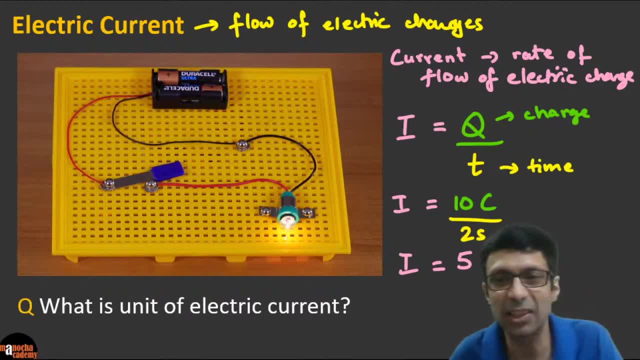 Sorry, of electric current, So it's coulombs per second. And excellent guys, You guys already have the answer. this question, Right? So what is the unit of current? It's basically ampere, Right? So you must have heard of this in your daily lives. 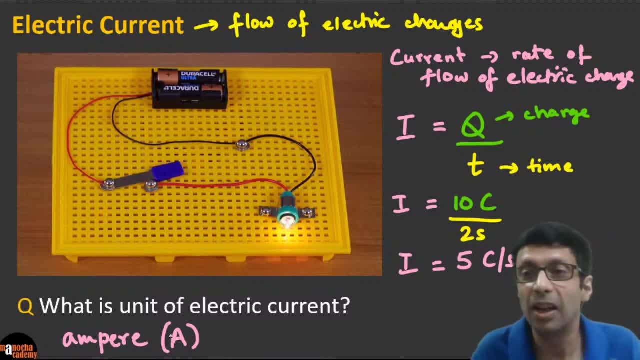 Right Five ampere, current 10 ampere. So this is ampere is basically nothing but coulomb per second Right. So coulomb per second has the symbol of ampere, So we can write: the current flowing here is five ampere. 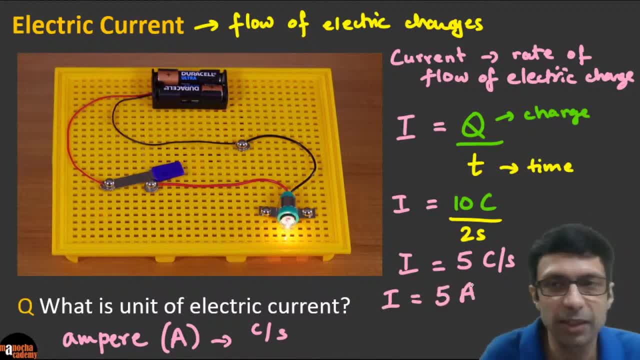 Very simple formula. You just divide the charge flowing, divided by the time, So 10 coulomb by two second, And that's going to be five ampere. Excellent guys, Clear So current electric current. remember that it is the rate of flow of charge and the symbol of electric current, as we discussed, is I. 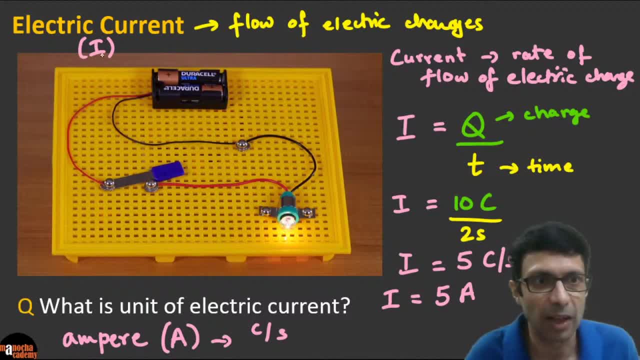 So there are a lot of symbols and terms to know in electricity And we can say: current is flowing in these wires And as we discussed what is flowing, the electrons Superb. Now question is: who is moving the electric charges? 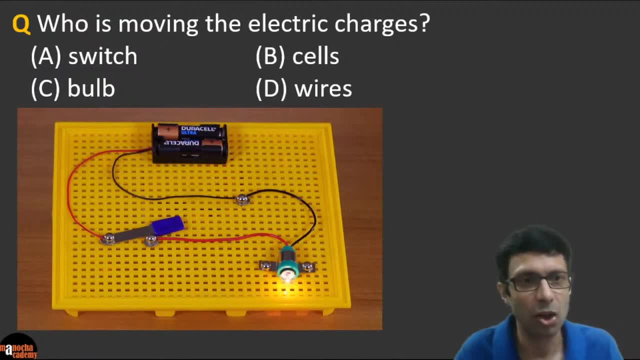 Right. So we said that the electrons are moving in the wire. So I have this question, guys: So in this circuit, right, So in this setup of the you, you can see the cells are there, the switch, the wires, the bulb, right? 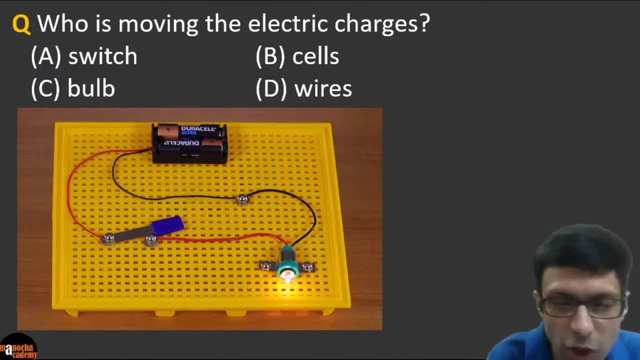 So can you tell me who is moving the electric charges, or in other words, who is moving the electrons Right? So what do you think? Is it the switch, the cells, the bulb, the wires? Come on, I want all of you to try. 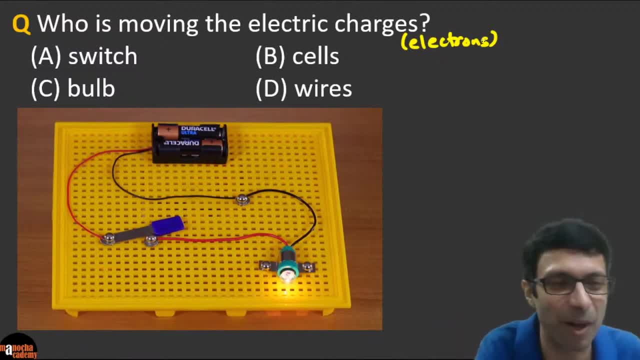 And I want all of you participating here to also hit the like button and share it out with your friends so that we can have more people on these live classes. So come on guys. Okay, Very good. Some are saying cells, some are saying wires. 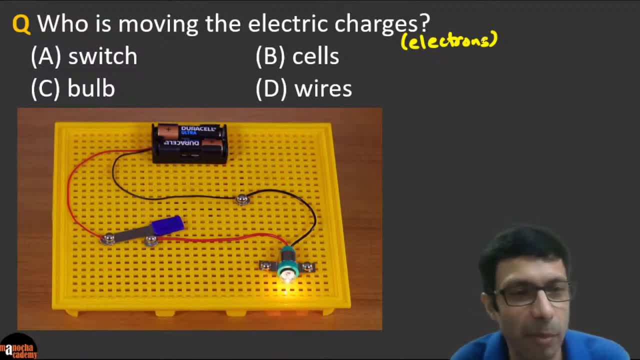 So come on, What do you think it is? It's excellent to see the response of everybody trying here. Very good guys, Very good. So electrons are flowing, But my question is: who is moving right? Who is pushing the electrons? 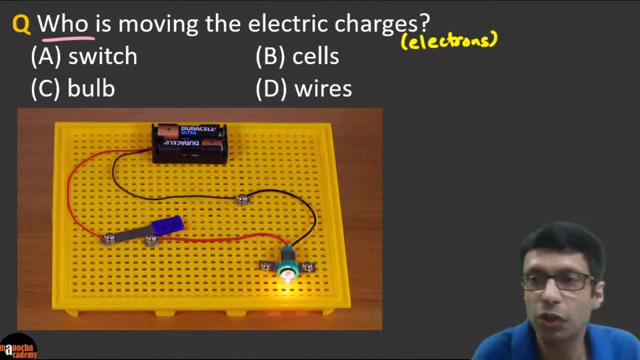 Okay, So you know it can't be the switch, right, Because the switch can go on and off. So this answer is definitely not the right answer. Okay, And it can't be the bulb also, Right, Because you could have a fan. 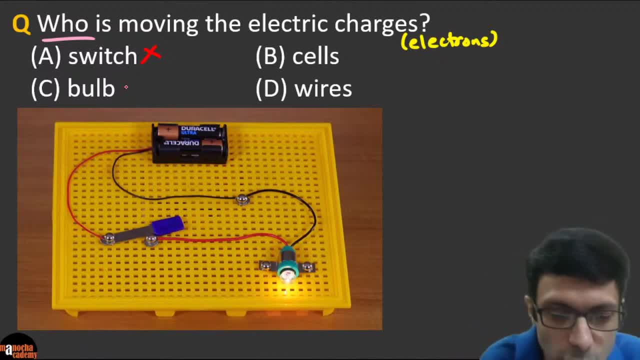 You could have a different electrical appliance, So you just don't need a bulb, Right. So that is definitely wrong Wires. So definitely we said electrons are flowing in the wires, Right. So if we draw these electrons right, So let's say there are these electrons in the wires. 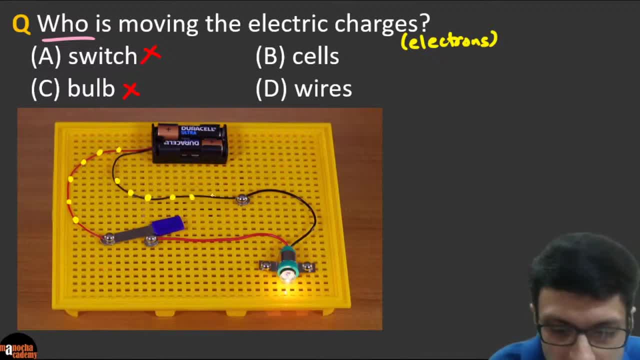 Okay, So I'm drawing these electrons with the yellow dots here, Right, Can you see, Right? So electrons are flowing in the wires Right, There's a continuous motion Right, And we'll talk about the direction later. Okay. 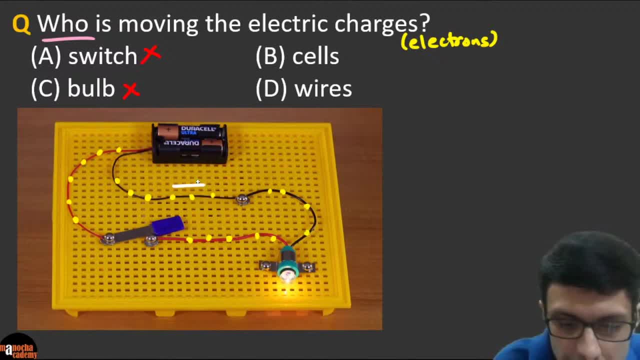 Right. So let's say the electrons are flowing this way in the wires, Right? So now, who is causing it? Definitely, the wire is needed, But you know that a wire is not sufficient, Right, Because what do you need? Very good guys. 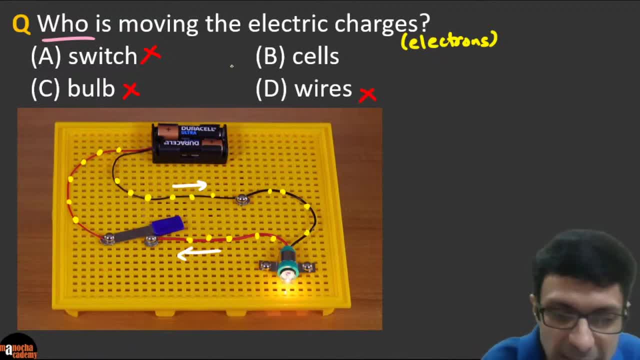 You also need a cell. So till you connect the cell or the battery, what we call, you will not have electric current. So very, very important concept, guys, It is the cells, Or what we call as a collection of cells here. 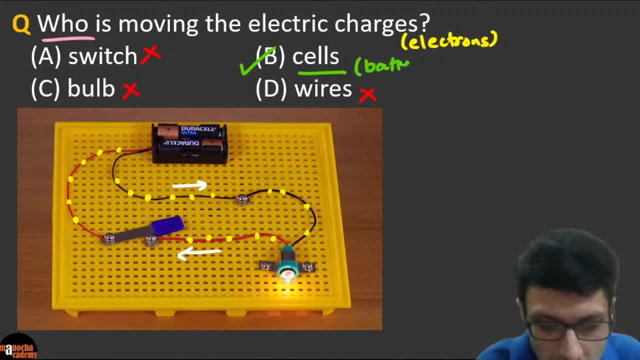 Can you see It's known as the battery here, So that is needed for the electric charges to move, or the electric current, And what is the general term used for this? So very important. So what is? cells or batteries, or you know the electrical supply that you're getting at home. 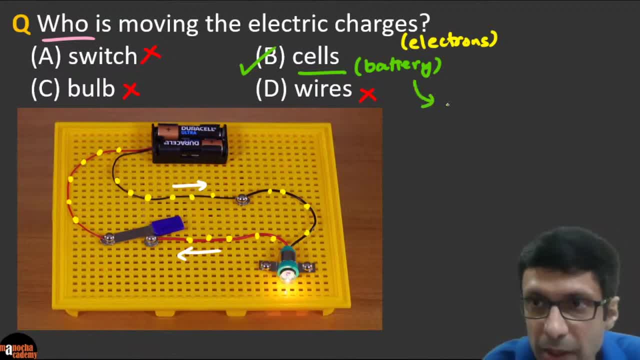 So what is that known as? So the general term is this is called as electric potential- Very important. So the term is electric potential, also known as voltage or also known as electric potential difference. There are many terms, right? So electric potential difference. 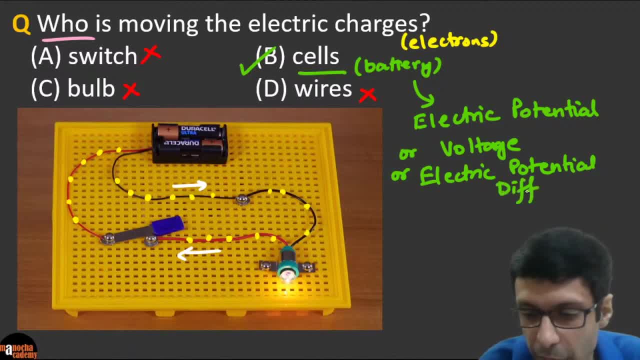 Right, guys? Or simply potential difference, Okay So. or let me write all those terms here for you, Right? So these all mean the same thing, Okay, guys. So electric potential voltage, electric potential difference or potential difference- So very important for you. 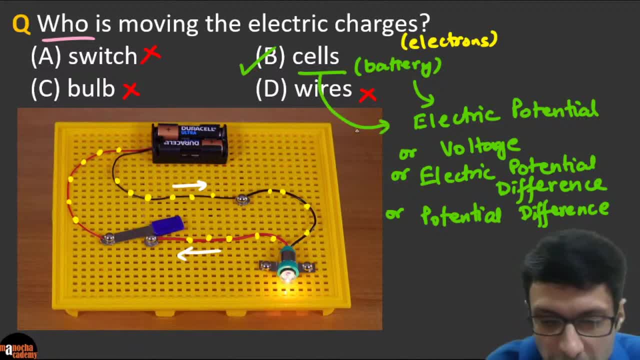 You know that cell supplies this electric potential, right? So cell is providing this thing, Okay, And it is the cell which is driving the electric current. So it's very important sentence: If there is no electric potential difference, or there's no electric potential, there will be no current. 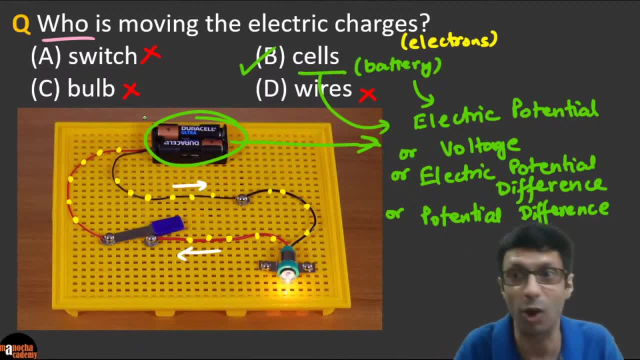 Okay. So if the electric potential goes in my house right now- I hope it doesn't- This live class will stop because there will be no electricity. My computer will not run, I will not be able to, My camera won't run. 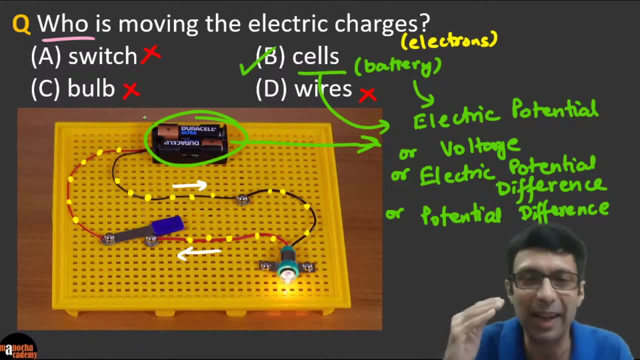 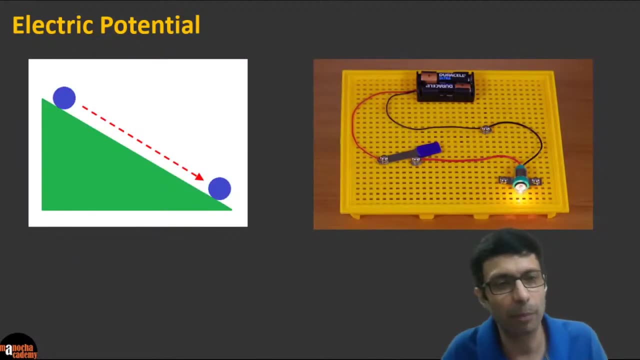 Nothing will run right in the room. So very important electric potential or electric voltage. Voltage is needed for moving the electric charge right Or for the flow of electric current. Very important concept. Now, what is this guy? So what is electric potential? 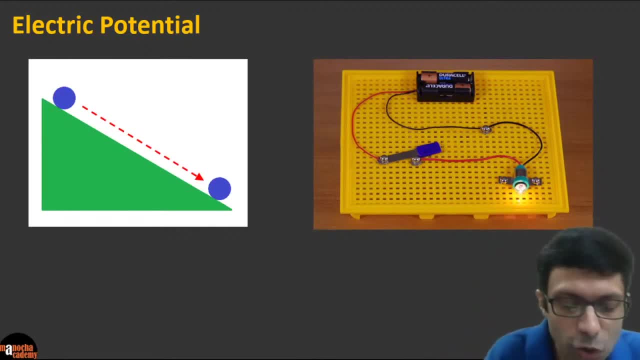 Let's understand it. So, guys, do you know what is electric potential? So you must have heard of this term, right? Potential energy or potential, right. So you need a potential energy or potential At a height, right? So you've heard of this term. 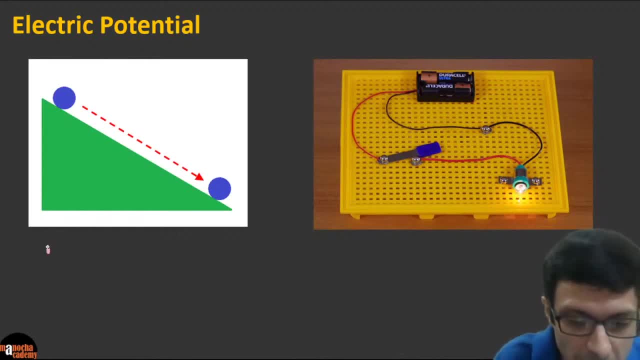 So let's write it here, right? You've heard of this term potential energy, So this term sounds similar, right? And what is potential energy? Energy at a height, Right? You've seen this. So can you see that we say that this ball has high potential energy when it's at a height, right? 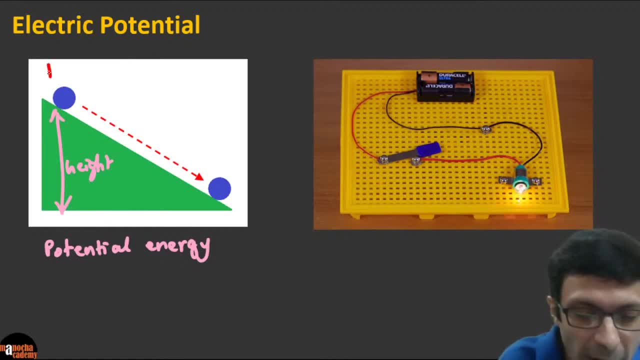 So here it's moving from high potential or high potential energy to low potential energy Or low potential. Let's write it as potential here, So I'll erase this and write Okay, So you know, for the motion of this ball right. 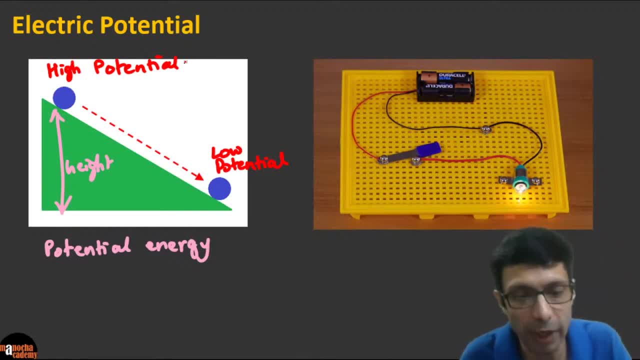 Right, You need a high potential to low potential. So what are we having here, guys? Very important concept. So can you see, there is a potential difference needed. So potential difference is needed for the motion of the ball. Potential difference is needed for the motion. 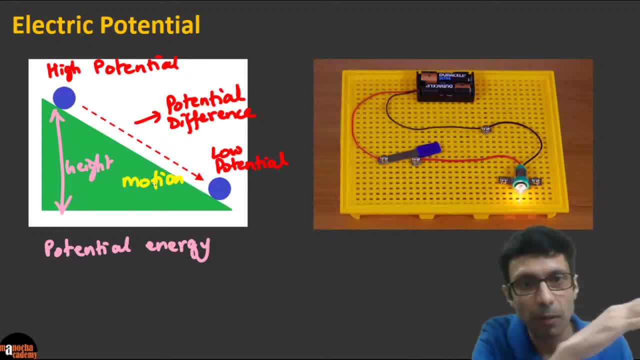 Similarly, you know that for water to flow, you need a slope, you need a potential difference, right? Water has to flow from high potential high potential energy to low potential energy. high potential to low potential- okay, So that is why we have the term potential, right. 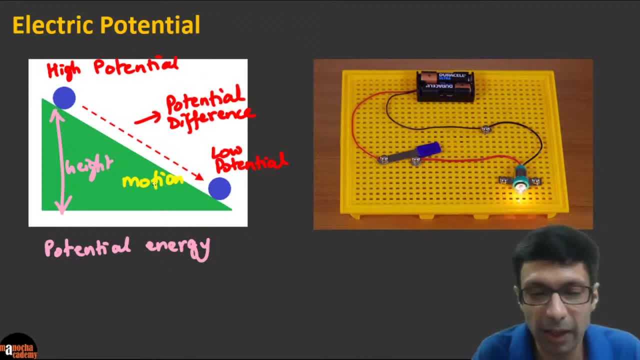 And similarly here, guys, okay, it's similar thing here, that electric potential is what we are having in electricity also, right? So electric potential is needed for the flow of charge. So you can think this: what is this electric potential exactly? You can think it like: electric potential is basically like electric pressure, right? 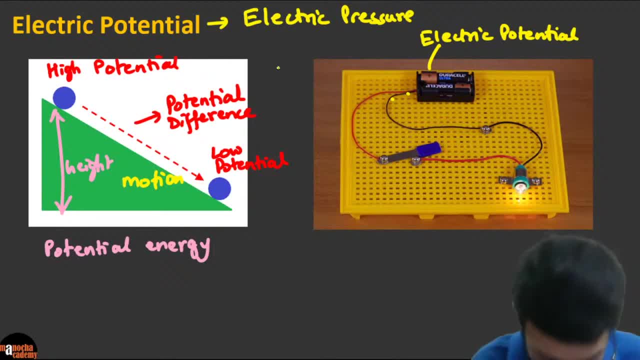 There's some pressure needed for the electrons. Let me draw the electrons- I think in white Look better here For the electrons to move. okay. So some electric potential is needed right to move these electrons. It's like a motor. You can think a motor is needed to move the water right to make the water flow, or a height or a slope is needed. 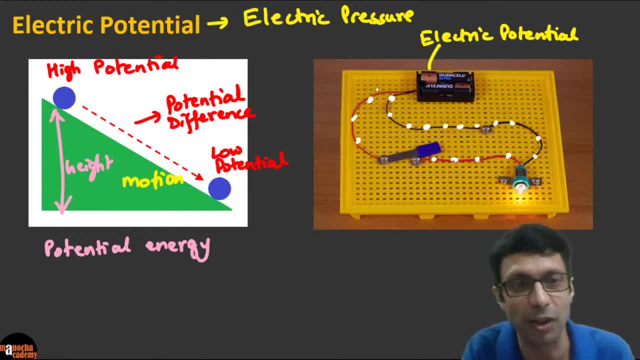 Similarly, electric potential is like an electric pressure that is needed to make the electrons move for the flow of charge right. And if you don't have that, obviously that bulb will not glow, You will not have Any charge. So you know, when the cells, the battery, run out, the electric potential will become zero, The bulb will stop glowing. clear, Very, very important thing for all of you to know: Electric potential is like an electric pressure. Just like you know that when the exams are near, we are under pressure to study- right, We study with the exam pressure. or if we have a deadline to meet some homework to do, we study because of that pressure. That pressure drives us to finish off our syllabus right. Similarly, it is this electric potential, or what is known as electric potential. 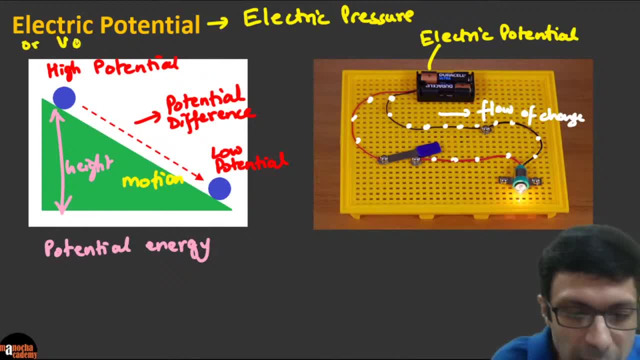 Voltage. Same thing, guys, Electric potential of voltage. It is like this electric pressure pushing the electrons, because if you don't push them they are just going to move randomly in the wire. There's going to be no current. Clear, Please clear your concept. This is very, very important. Excellent. And now how is electric potential defined? It can be defined as the So electric potential or electric potential difference, right, We say between two points, right? 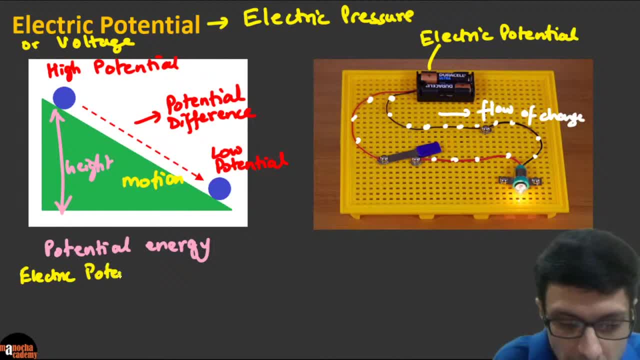 say, if you consider the electric potential difference between two points, it is defined as the work done. so let me explain that to you guys. so it is defined as the work done per unit charge. so what does that mean? so the formula is electric potential between two points. 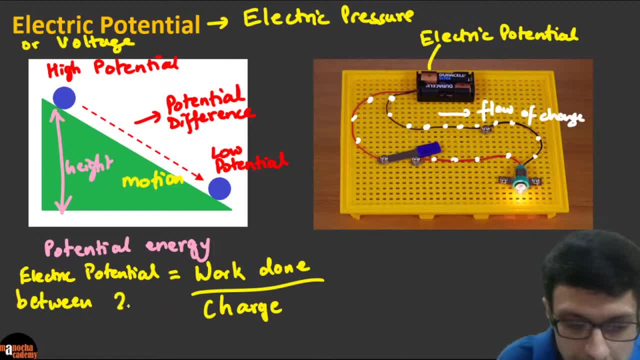 let's write that here: between two points. okay is defined as the work done by charge. so two points means any two points you're considering in the circuit. let's say this point here, point a and point b, right? so whatever two points you're considering, or the ends of the battery, right? 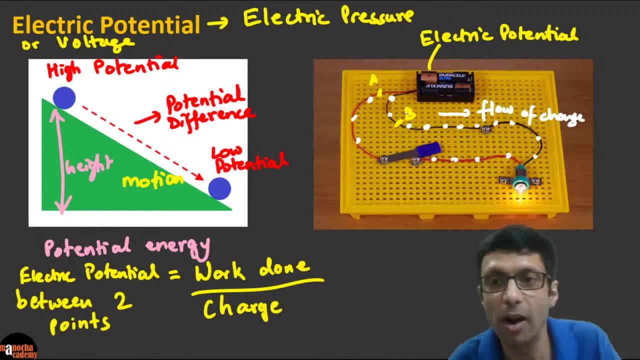 the terminals of the cell, right, so it is defined as the work done by the charge, right? so let's take an example. let's say the battery. here the cells are doing, let's say, 10 joules of work. okay, so they're doing 10 joules of work to move 5 coulombs of charge. okay, so the work done is. 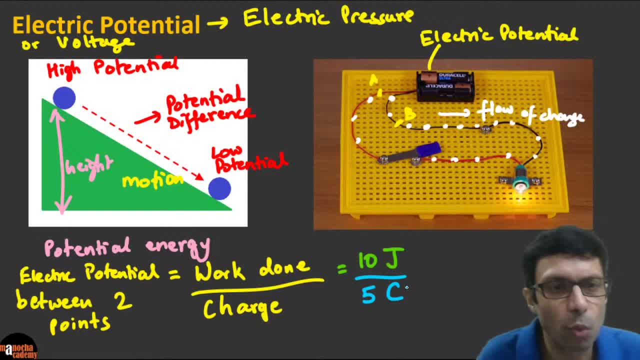 10 joules divided by 5 coulombs. okay, so what is the potential difference? come on, can you guys calculate? so what is the potential difference going to turn out to be? work done per unit charge means work done divided by charge. so who can tell me what will be the electric potential here based? 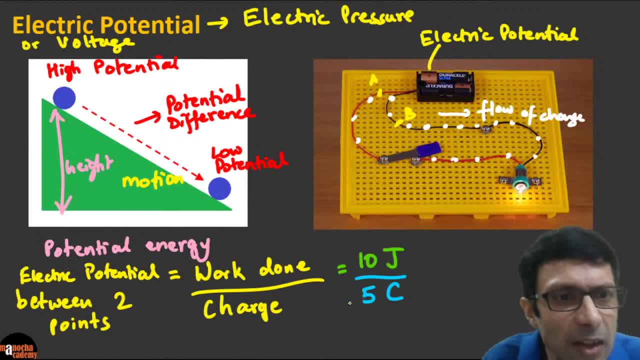 on these numbers. excellent, i see narendra has the right answer. uh, sridhar sharia. come on, guys, all of you think so. it's going to be 10 by 5, simple 2 joule per coulomb. right, let me write that in. 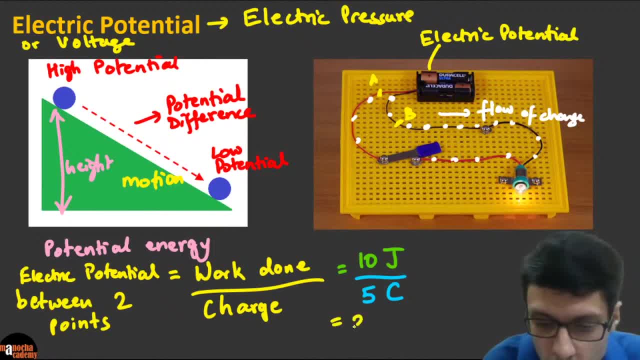 yellow here. so it's going to be 2 joules per coulomb, and this joules per coulomb is known as volts. okay, because the potential difference. so here the electric potential is going to be 2 volts. okay, so electric potential is equal to 2 volts here, because joule per coulomb the si unit is. 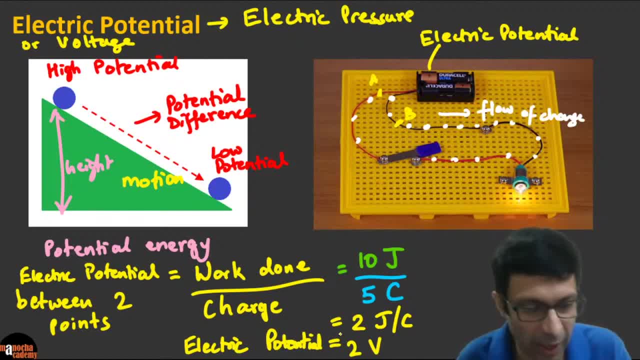 basically volts clear. so that is the si unit of electric potential right joules per coulomb right, and we do, uh, we have 10 joules per 5 coulomb. and who's doing the work? guys, the work is done by the cells. here they are doing the work right. 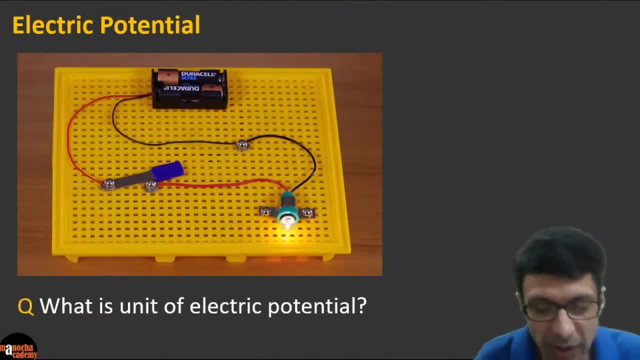 is that clear? okay, so that is the important thing here: that electric potential is the work done by these cells, right? so who's doing the work? these cells, very important for you to remember and as the unit of electric potential we just discussed, guys. so can you tell me what is the si unit? so, unit? 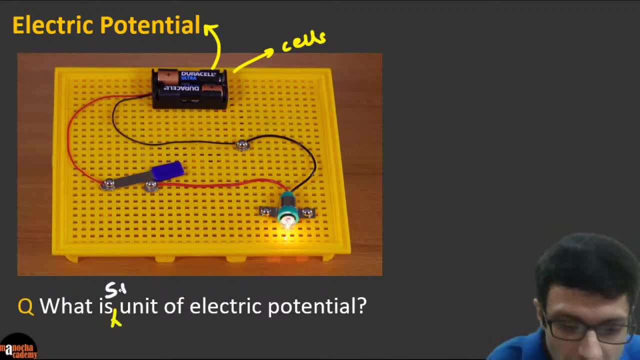 means obviously we are talking about the si unit here. what is the si unit of? electric potential volt? very good, very good. so the si unit is going to be volt and the symbol is basically capital v. okay, so, guys, please remember that. and potential difference. let's again write the formula clearly. 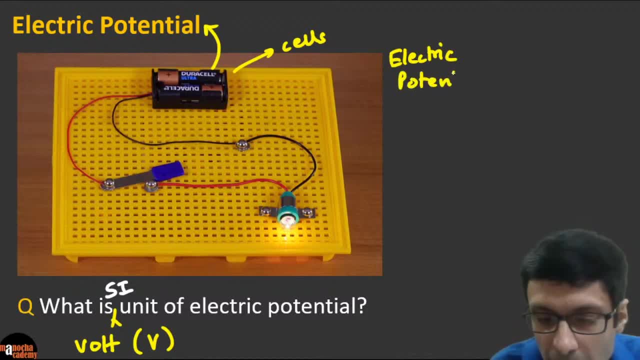 electric potential is basically work done, right, so you have work done by charge per unit, charge- very important formula, okay, and that can also. you can write that down as w by q, okay, guys, so electric potential is w by q and the symbol for potential also is v. so the symbol for electric potential is also v, just like the 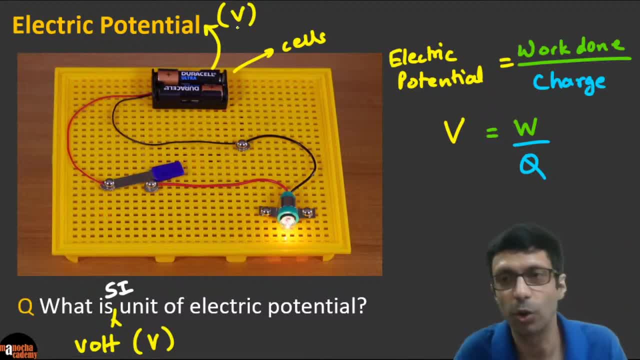 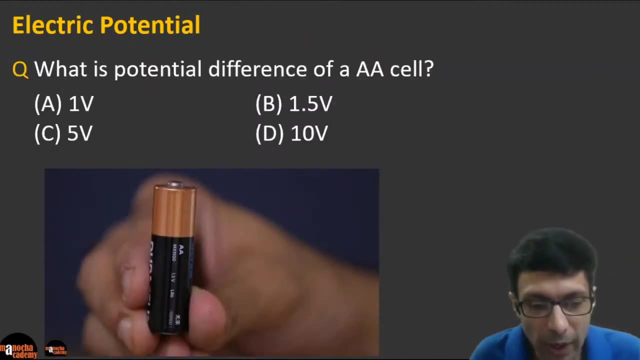 symbol of the si unit is v, for volts is v. okay, so v is equal to w by q. clear guys, okay, so we're talking about the potential of the potential difference in the potential difference in the potential difference between cell and battery, and these cells are known as a cell. 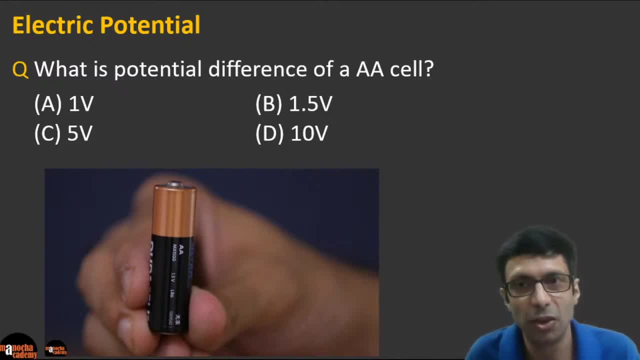 right. okay, and please understand what is the difference between cell and battery. battery is a collection of two or more cells right. so typically when you have one like this, we call it cell right. battery is typically two or more cells right and cell says that you need to have a say, that you need to be paid. so that means if you want to have a data to see. 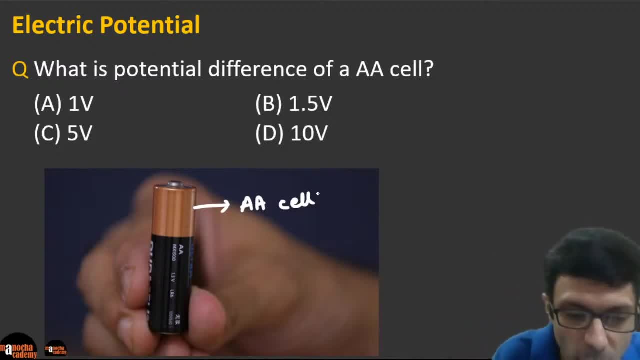 more cells. So who can tell me what is the potential difference and what are we measuring? the potential difference between these two points, between the positive terminal and the negative terminal of the battery. Potential difference means it is measured between two points. okay so, and potential difference is: can be measured using a volt meter. okay So, just like current. 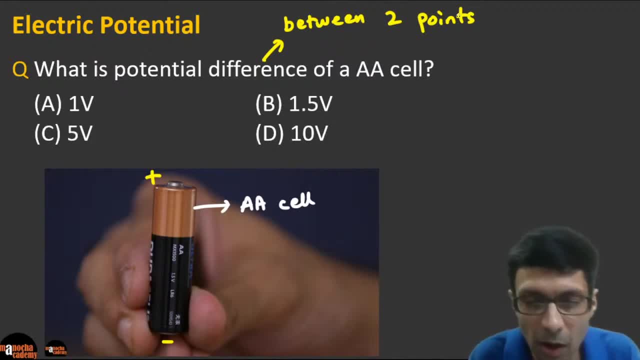 I think I forgot to mention current. you guys know can be measured with an ammeter. Potential difference can be measured using a volt meter. So very good, I am seeing different answers here. so potential difference can be measured using a volt meter. it is an instrument, right? So if we 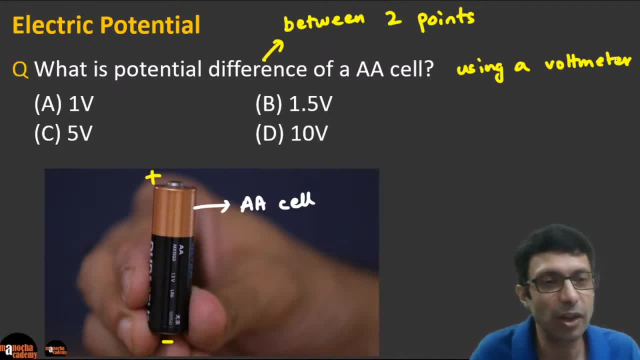 connected a volt meter to this cell, right, how much electric potential it would be right. and, guys, if you have a cell at home, please pick up and check, right. I think I do not think you can read it here. it is really written in small. the value is actually given here in the picture. the correct answer is: 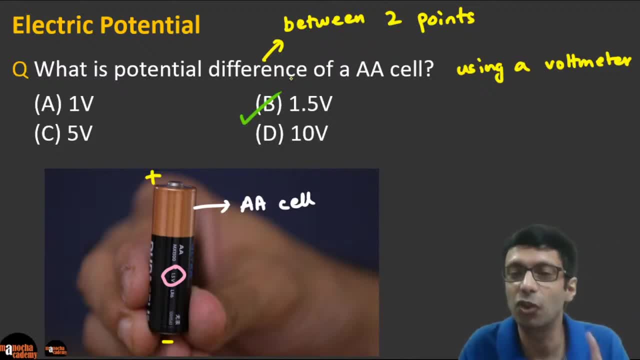 1.5 volts. please check Even a AAA cell, the thin cells, the AA, AAA, they are all 1.5 volts each, typically right, So absolutely very good. some of you got it right. So the electric potential or the voltage that this cell can supply. 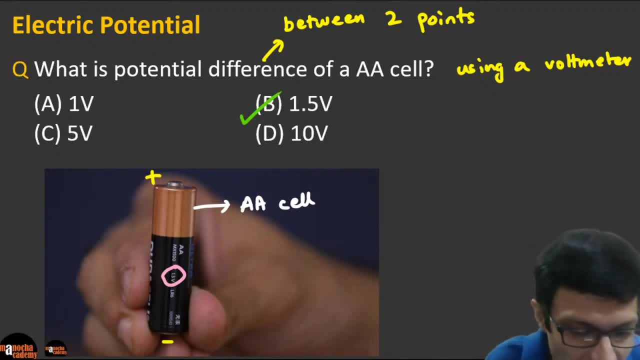 is 1.5 volts. awesome, correct answer, fantastic guys. So please remember, and I encourage you to pick up a cell at your home and do check the value. you will see it is clearly written there: 1.5 volts. and remember Volt is the unit of electric potential. the guy who is doing the work, the guy who is pushing the 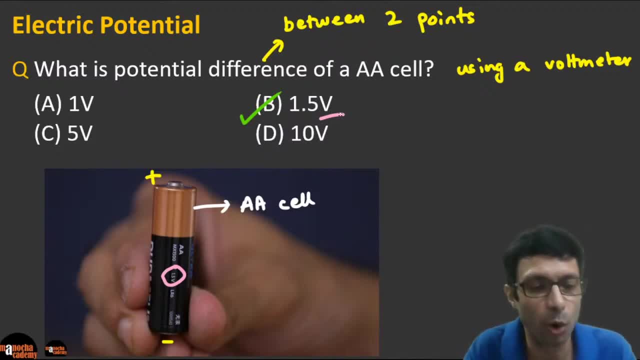 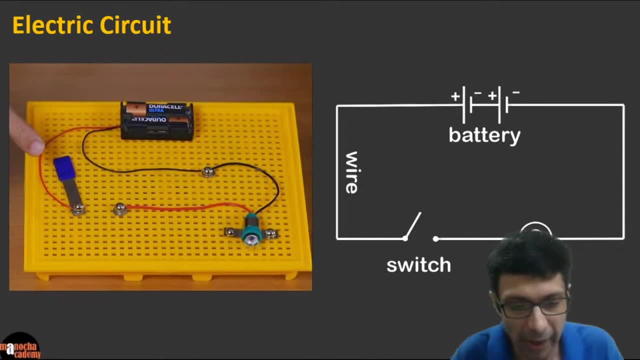 electrons in the circuit, the guy who is responsible for the flow of electric charge? awesome guys. Now let us talk about this concept of electric circuit. so we talked about electric charges, we talked about electric potential. now let us also talk about electric circuit, guys. ok, So here you. 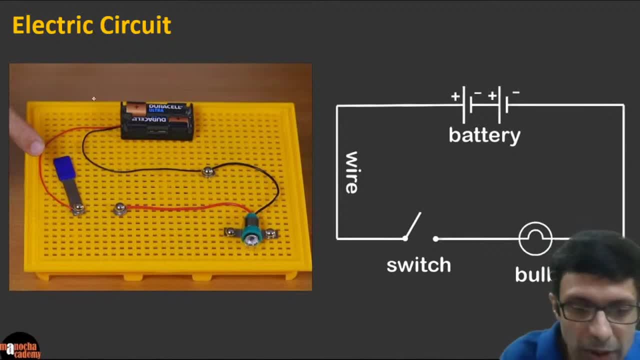 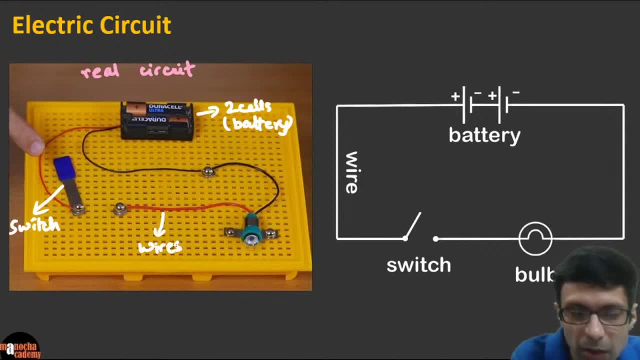 These are, of course, the wires right, and here you have the small bulb, Right, guys. so this is the real circuit and here is what we draw. this is known as the circuit diagram. I am sure those of you who are doing electricity- I know a lot of you- are doing it, because that is why you requested for this electricity class. so here we are discussing the awesome topic of electricity and this is a circuit diagram, which is a simplified diagram, right so, where we use circuit symbols. so you can find this in the book and you will see that. 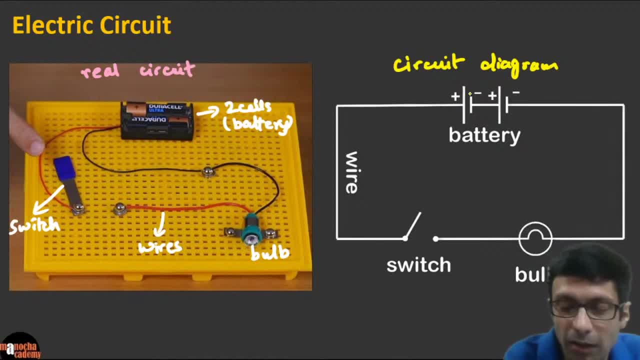 This is the. This is the symbol used for batteries. where this is, each one is the individual cell. right, so this is a cell. so can you see there are two cells drawn here in this battery, right, so there are two cells and they are marked with a plus- minus. right from that shows the potential difference, right? so plus is the higher potential difference, positive potential difference and minus is the lower potential difference. and all these lines here that you see, these are the wires, right and wires you know they are good conductors of electricity. 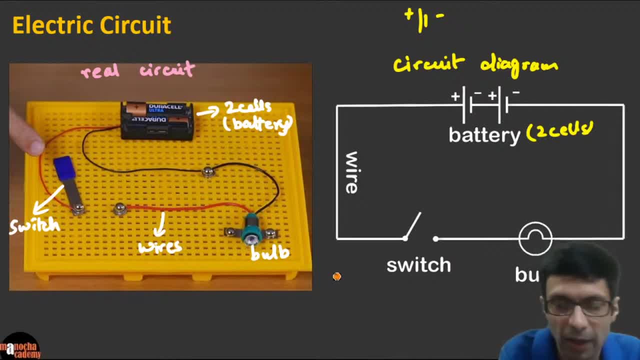 Because the Electrons can easily flow in the wire. and then here, what you can see here, this looks like a gate, right? so this looks like a gate. this is our switch. so when the gate is in the open position, the switch is off, and when you close the gate, the switch is going to be on, okay, so, guys, this is known as a. so when the switch is off, so very important thing- when the switch is off, it is called an open circuit, right, guys? so switch off is called open. 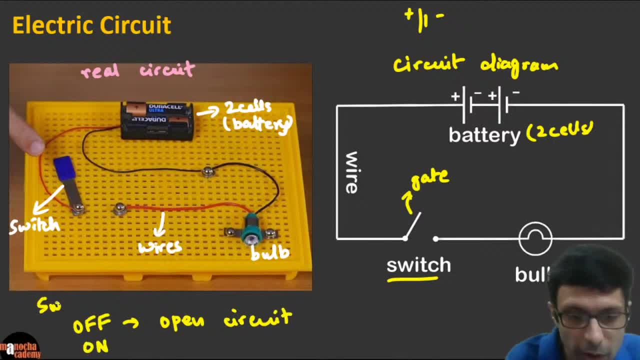 Okay, And when the switch is on: okay. so when we are talking about the switch on off, it's known as a closed circuit, right, because the gate is closed, so it's easy to remember. so closed circuit is when the current will actually flow, right, so if I want to close this circuit, this will no longer be there, so we will cancel this out and we will draw the line now like this: you guys got it. so now this is going to be a closed circuit and the current can flow and the bulb will start glowing here. this is the symbol for bulb there. 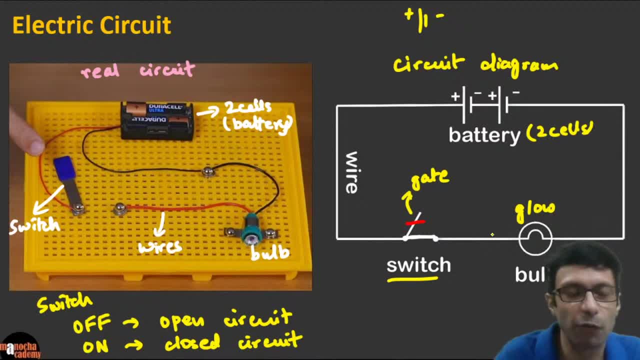 There are other different symbols which you can learn, so this is not the only symbol for a bulb. okay, guys, so this is known as a circuit diagram, which is a simplified diagram of this circuit, because every time you don't want to draw this actual thing, right with the bulb and the batteries, you will draw a simplified diagram. like this can all of you see- and very good, I see some of your writing- the closed path through which electricity can flow is called an electric circuit. excellent, guys, so this whole setup, or the closed path, 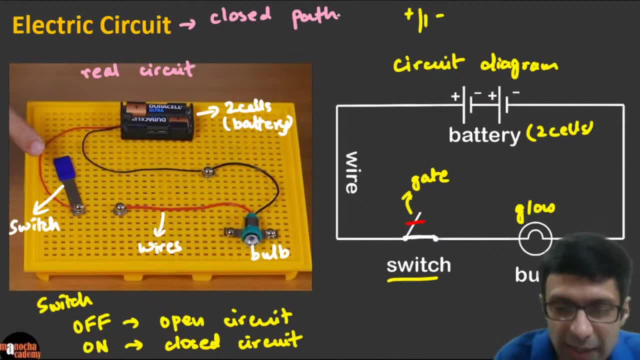 Through which electricity flows, is called the electric circuit. this entire setup here, right, so, this entire setup which contains the cells, the wires- cells basically means potential difference- the wires, the conductors through which electricity can flow, the switch, the bulb, this entire setup is known as an electric circuit. okay, clear guys. so, and this is a circuit diagram, you must practice the circuit diagrams, draw the wires and always remember to mark the positive and negative potential. 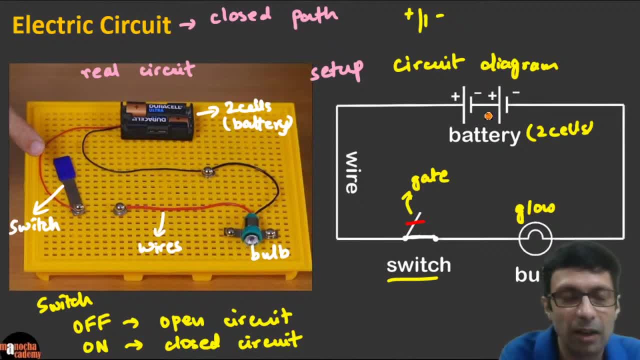 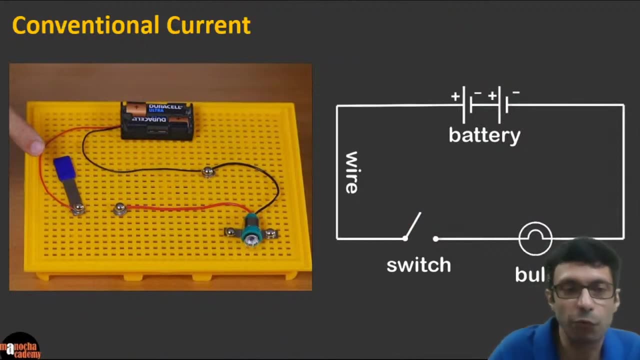 In the Battery, because you know the every, everything has the cell. it has a plus and a minus right potential. okay, excellent guys, is that clear? now let's, we didn't talk about a very important thing, which is going to be: what is the direction of the flow of current? so I told you we'll be coming to that, right, guys, because the we know that the electrons are flowing in the wire, right, did we discuss about that? so, because we said that when this circuit is going to flow, 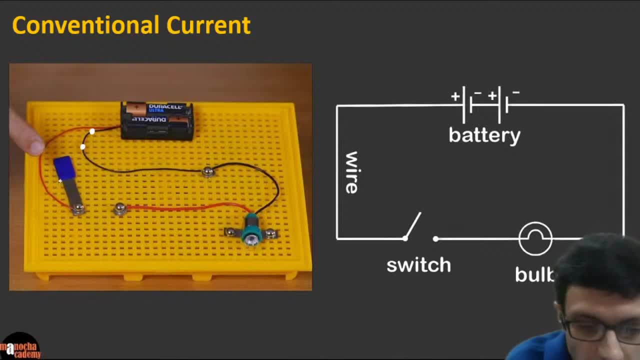 So This is on right. so when let's say the switches in the on position, so let's say we cancel this and the switch becomes here in this on position. so when we switch, switch it on here, right, then these electrons are going to flow, Right, so the electrons will start flowing in the wire, okay. so one very important thing is, guys, what is the direction of flow of electrons? excellent, I see nippon is already given an answer. raja mukherjee is trying an answer. excellent, guys. so 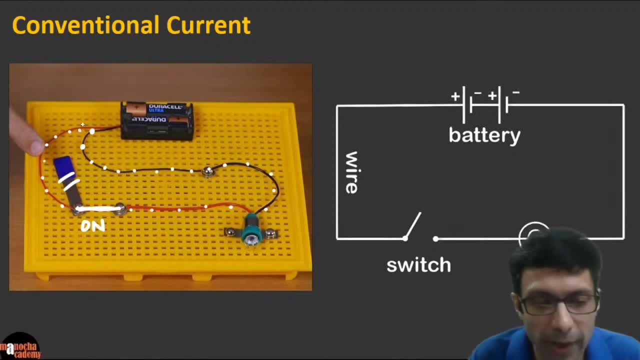 Guys, Think, what do you think will be the answer here? so when electrons are flowing in the wire, right, what is the direction of flow of electrons? because you know that when you connect this the electrons will be flowing. Right, so electrons are flowing, But what is the direction of flow? so I'll give you two options here. so you know that the cell has, you know, the positive and negative right. so it has a positive terminal and a negative terminal right, this battery. so can you see here, guys, 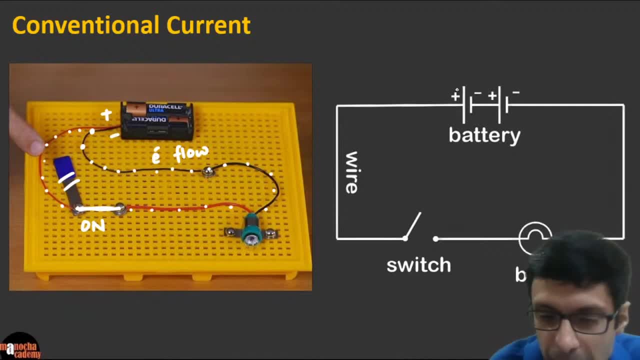 This is the positive side. can you see on the circuit diagram- I'm marking this in pink here on the circuit- and the negative here can you see in yellow right. so this overall, there's a plus minus, right. so now the question is: are the electrons flowing from positive to negative or negative to positive? very, very important thing to know, okay, what is the direction of flow of electrons? so how will you remember this? let me share a very simple technique, a very simple tip for you. you know that the electrons are 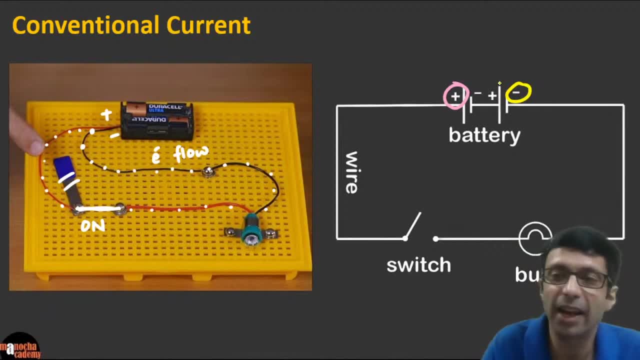 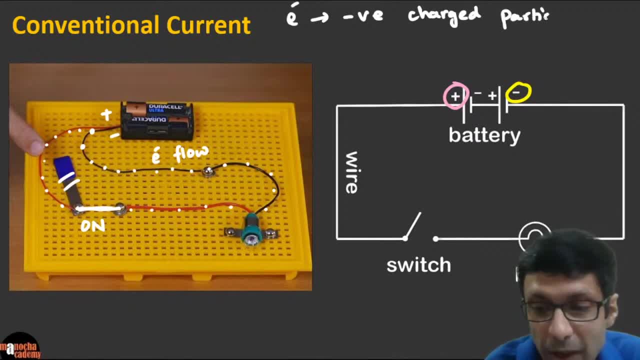 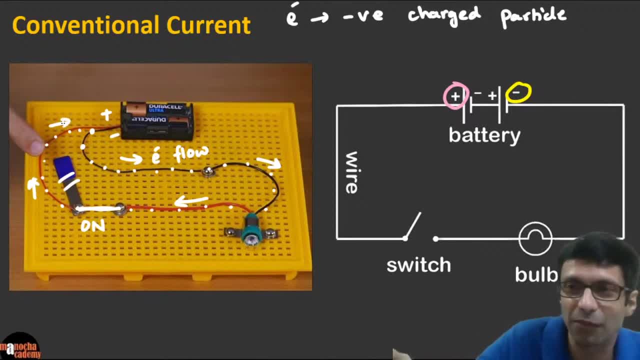 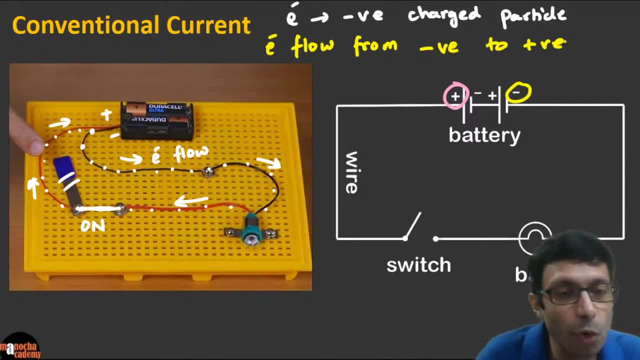 this current known as- so we know it's called electric current. so the flow of electrons, the direction of flow of electrons, this is called electronic current. very important term, electronic current. okay, so if we mark it in the, let's mark it in the circuit here. right? so let's mark our electronic current. 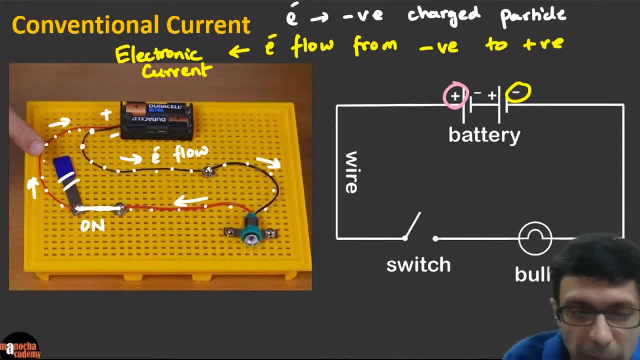 what direction it's going to follow. in the circuit it's going to be this way, right? so the electrons are flowing from negative to positive. so electron flow- if I'm marking, please note I'm writing the E over there, right? electrons are going to flow from negative to positive, of course, when the switch is closed, right? so let's. 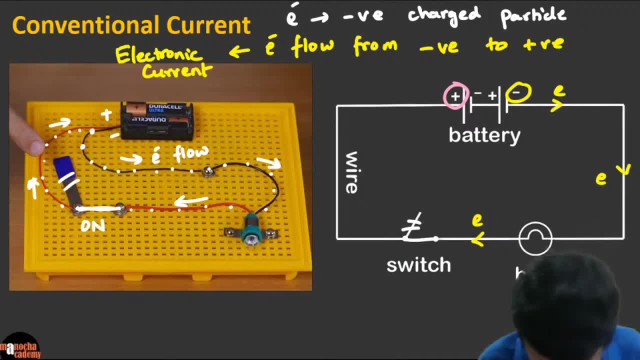 say the switch is closed here. right, let's cancel that in red here, right? so let's say the switch is closed. so the electrons are going to flow from negative to positive, right? does everyone agree? this is known as E represents the electronic current. okay, but now there's one very interesting thing, guys. do you know there's another? 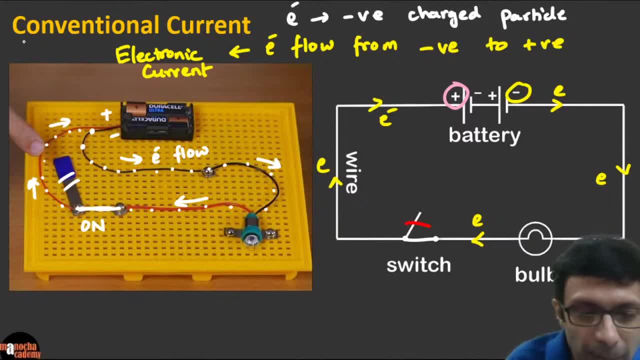 term. right to make things confusing, there are a lot of terms in electricity, that there's a thing called conventional current. okay, so actually when you see the circuit diagrams, guys, the electronic current is usually not marked. okay, very important. so I'm going to erase this electronic current, or later we'll erase. 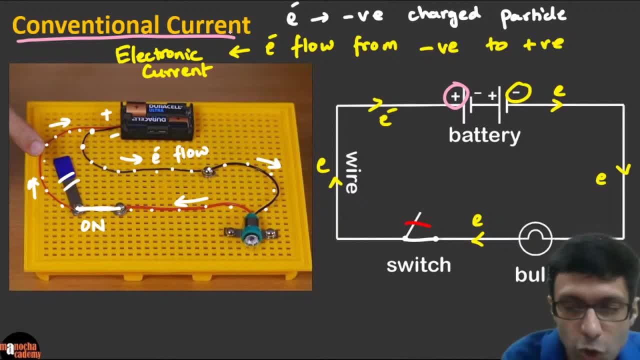 that later, right? so actually you'll find the current shown in the circuit, right? the conventional current is marked this way. so when they mark the current, it's from positive to negative, and do you guys know whyright? so the current in the circuit which I'm marking with the pink color and I symbol, right, I represents 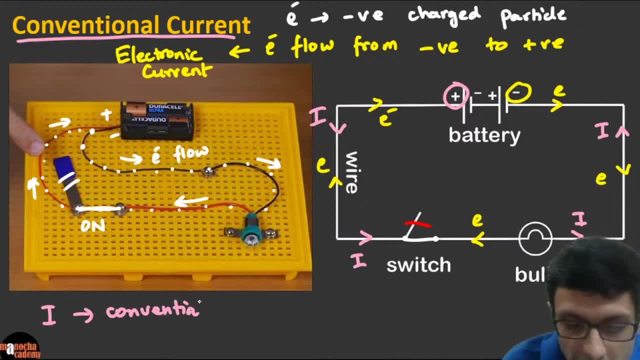 the conventional current. so I is conventional current, which is from positive to negative, positive to negative. okay, can you see in the circuit I've marked it for you, right? okay, I think my recognize that the circuit is marketing for you. use I before this to see walking back. actually, where am I there in the treatment? 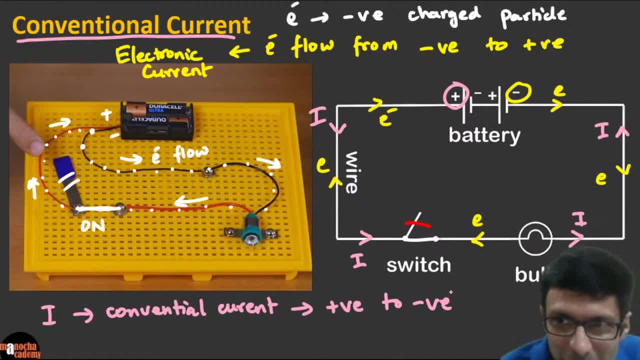 meal. same method, if you tell me the daher corruger intraoculardade. I've marked it so by. I think my head is hiding the circuit, so I am trying to dodge here. right and guys, the electrons, electronic current, which is marked with the E, is from negative to positive, So they are opposite. So question is: why this confusion? Which one should we use, guys? Do you guys know? 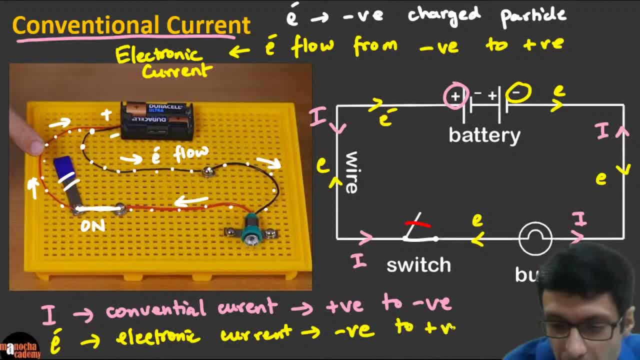 So electronic current is from negative to positive. Okay, So please remember that it is the conventional current that is marked. It is conventional current that is important, and it is usually marked from positive to negative. So why this whole confusion? right, The fact is because electric current was discovered before electricity, before the electrons. So electricity was discovered before the discovery of electrons, And when they discovered electricity, the 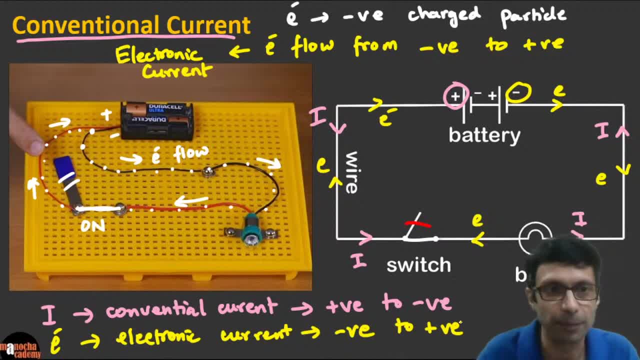 scientists assumed that it is the positive charges that are flowing. Okay, So they took that as the convention, just like they took the convention of, you know, a positive and negative charge for the glass rod and for the silk cloth and the ebonite, right? Those are all conventions. So same way that they made up right. So same way they said: okay, the electricity we are going to mark, just like water flows from high potential to low potential, We are going to mark electricity in the same way, from high to low potential, So positive to negative, Because electricity 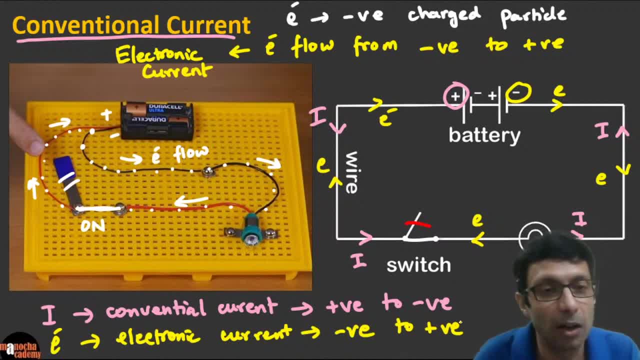 was discovered before electrons. But when they discovered the electrons they said, oops, it is actually wrong. The charged particles that are flowing in the wire are not positively charged particles. They are not the protons, because protons are tightly bound in the nucleus. It is really the light electrons that are moving in the wire, Okay. So they said, okay, that was wrong, but we are still going to. we are not going to change all the textbooks, We are not going to change all the scientific papers. We are going to consider the 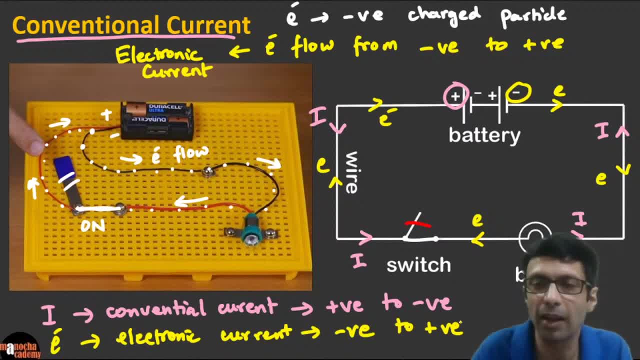 that as conventional current, because it is convenient to think electricity flowing from high potential to low potential, Okay, But the reality, guys, is it is actually opposite the electrons. But do not confuse. whenever you have to mark. So I am going to erase the electrons in that electron direction in that circuit, because whenever we mark it, guys, we always mark, unless really asked. we mark the conventional direction. So, guys, you can see I have erased the electrons. 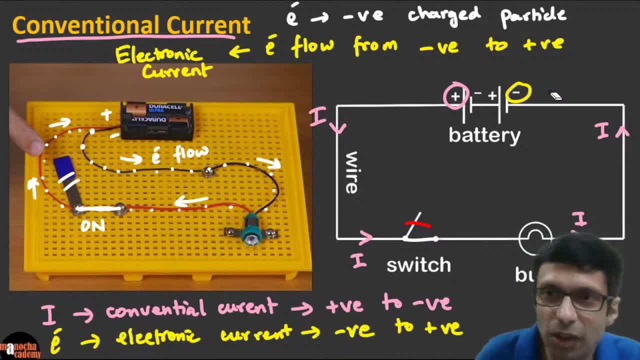 Okay, So please remember this very important concept: Conventional current is what is often marked, and it is from positive potential, or high potential, to low potential, and the electronic current is opposite. Okay, guys, So very, very important thing, Right, And it is battery, the cells, which is providing the. So let us revise that. So what is the cells providing the batteries providing the potential difference? So this is the electric potential, Right, Which is causing the electrons. 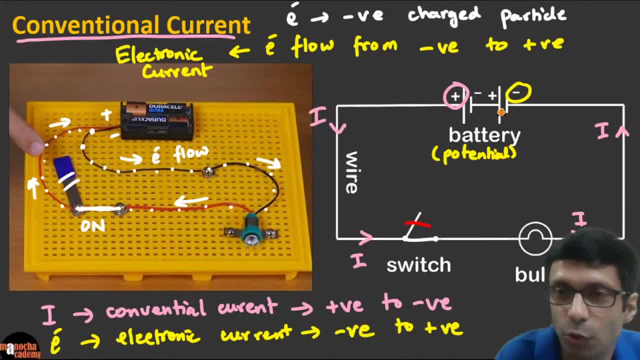 electrons to flow, or we think it the conventional current to flow from positive to negative, and that is why the bulb glows, Clear guys, And the wires are good conductors, you know, because wires are full of free electrons. So we'll not do that detail in today's class. 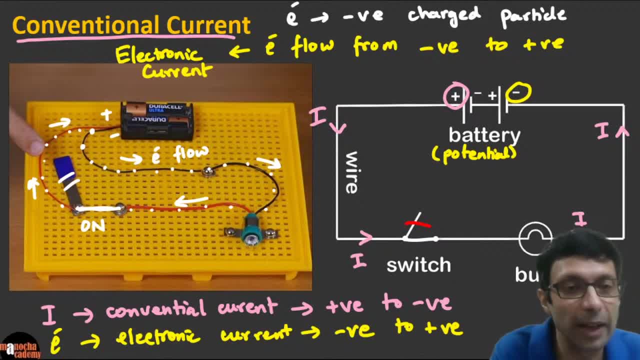 but wires are good conductors because they're full of electrons that can easily move in the wire. and who's pushing them? The electric potential, the battery, Clear guys. And so always remember to mark the conventional direction of current, Excellent, excellent. So, guys, I have one, 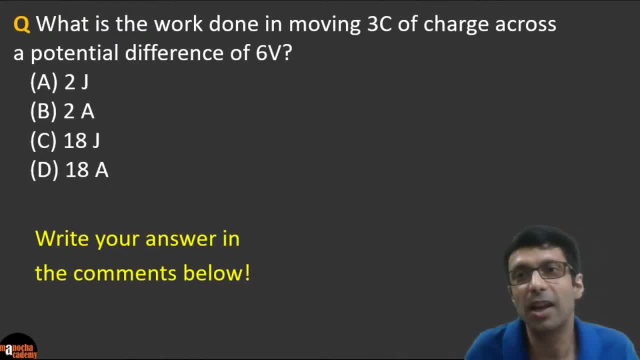 interesting homework question for you. What is the work done in moving three coulombs of charge across a potential difference of six volts? So you need to calculate the work done in moving three coulombs of charge across a potential difference of six volts. Is it two joules? 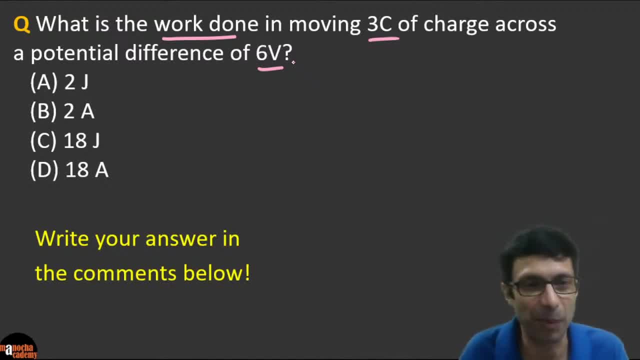 two amperes, 18 joules or 18 ampere, And guys do write the answer in the comment section below. I look forward to reading all of your answers and so please write it in the comments and I will promise to reply to them as soon as possible. So guys do write down the answers. 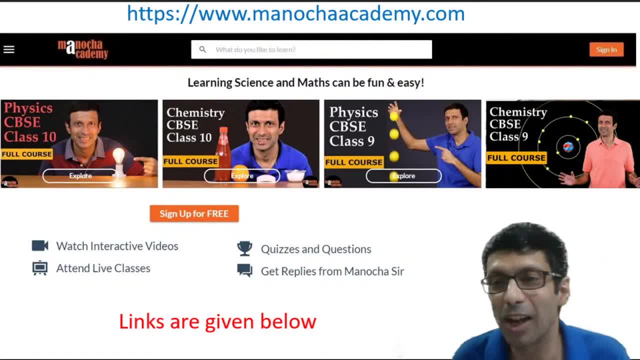 and thanks again for joining us in this live class on electricity. Hope it was an electrifying class for you and if you haven't subscribed to our YouTube channel, please hit the subscribe button right now and do click on the notification bell so that you get notified about more live. 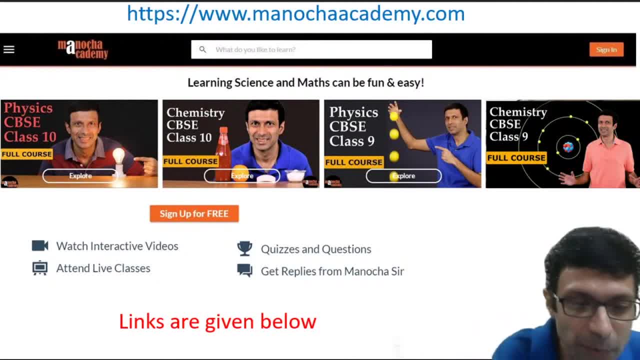 classes and the videos that we upload. And guys do check out our website because we have these awesome courses where you get to watch interactive videos. attend more live classes that I take on our website. There are quizzes and questions and you get direct replies from 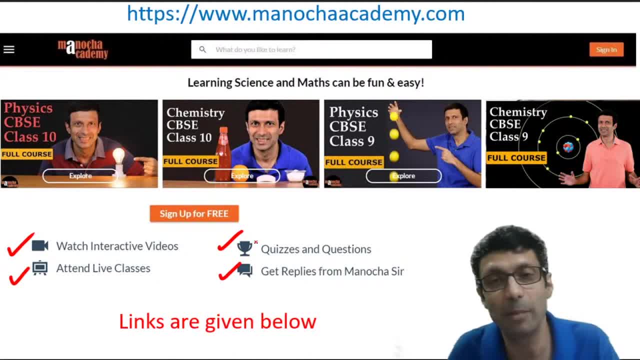 me. So, guys, these courses are at a special discount for a very limited time. so please do check out the courses on physics, chemistry and we have maths also launched for class nine and ten for CBSE board, and we have physics, ICSE, class nine for the ICSE board. So if you 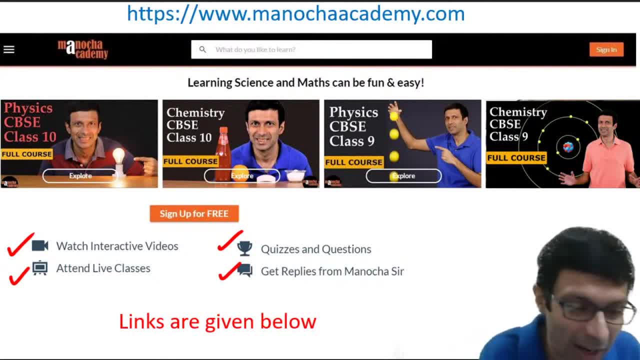 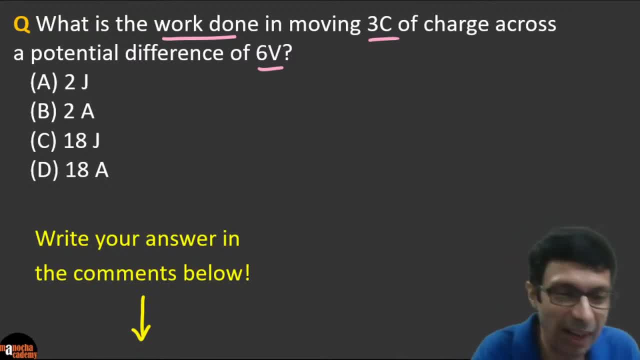 are interested in learning more about physics, chemistry, and we have some other videos that you can watch, so do check them out. Okay, guys? so do check it out and try this homework question and also you should find out that guys we talked about. remember I told about the cell, right? so do check out the cell. 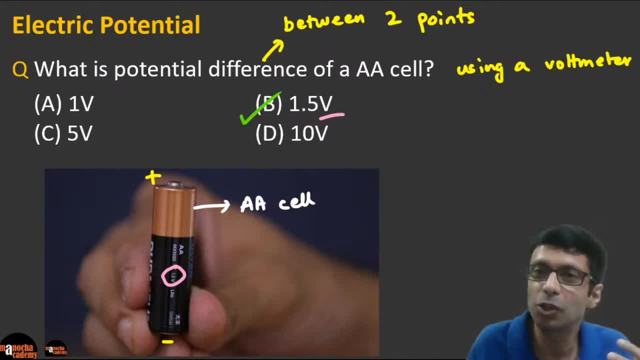 right, it is 1.5 volts, and do you know how much electric potential? so let me ask you: how much electric potential do you get at home? So what is the electric potential that you guys get at home, Do you know? So what is the voltage supply that is present at our 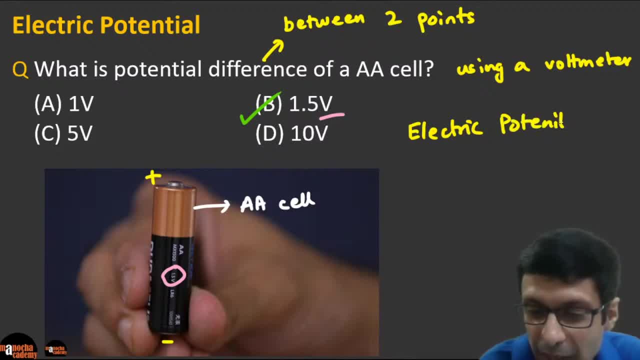 homes, electric potential that we get. so the electric potential- let me spell it correctly- a potential at home. okay, so how much are you guys getting? very good, very good. i see a lot of answers. so excellent guys. so in india you know the voltage is 220 or 240. so in india we write 220 volts, right? 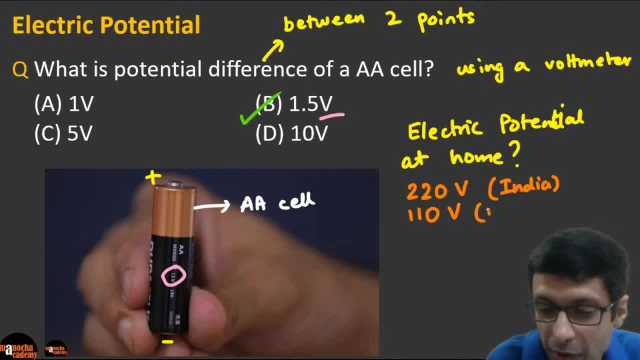 in the us, you know, it's 110 volts, okay, so different countries, they have different voltage that you get at their home, okay, so it depends on which country you're living in. okay, in india it's 220 volts. in united states of america it's 110 volts, i think. england, japan, they have a different. 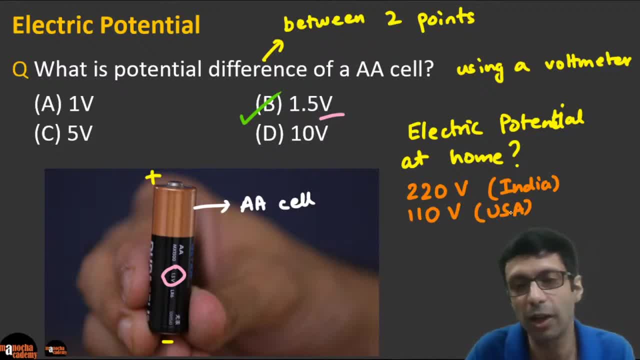 voltage. so, and yeah, of course it's a range 220 to 240. some somewhere it's written 230, but the standard value is 220 volts. so it's much higher than a cell, and that is why electricity is dangerous, because high potential can cause high current. you can get a very bad shock, so you should always be 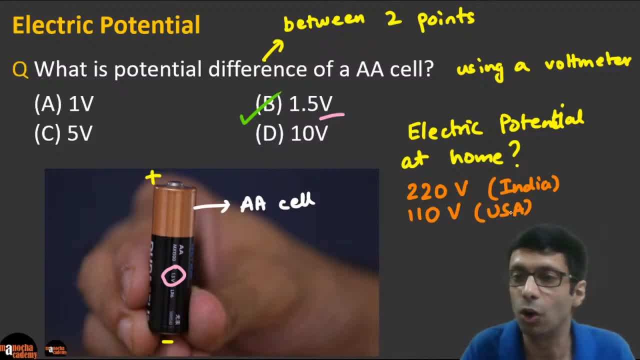 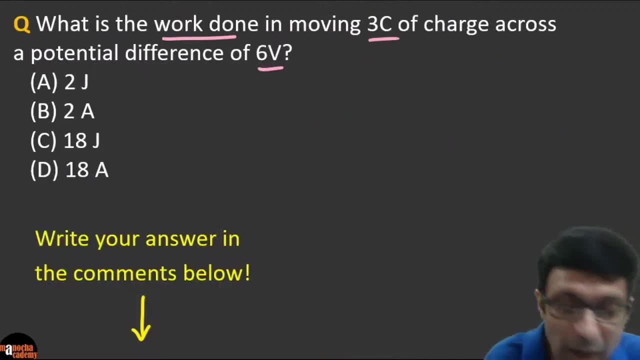 careful when handling electrical equipment. wearing your um, wearing shoes or slippers, right so rubber slippers, rubber shoes, okay, and never to touch switches with wet hands because there is high voltage coming in at the home. okay so, great guys, it was a great session. i really enjoyed it. you. 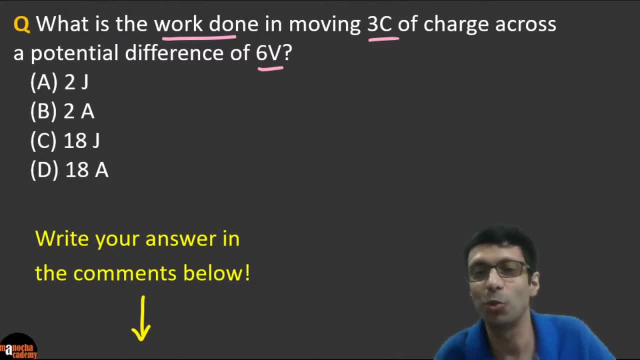 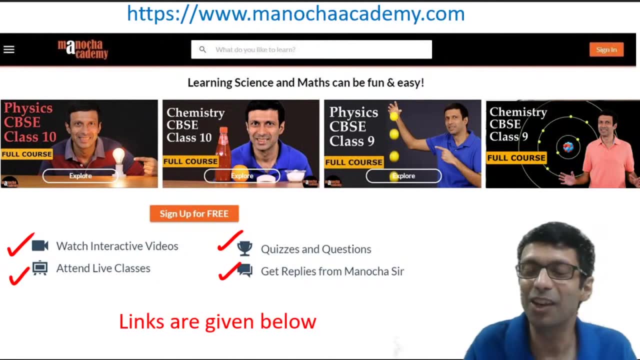 were really interactive. i'll not give the answer of this question because i wanted to put it in the comments below, and do keep checking our website and our youtube channel and, guys, if you haven't hit the like button, please hit it right now and do share it out with all your friends and your family, and thanks for joining us. 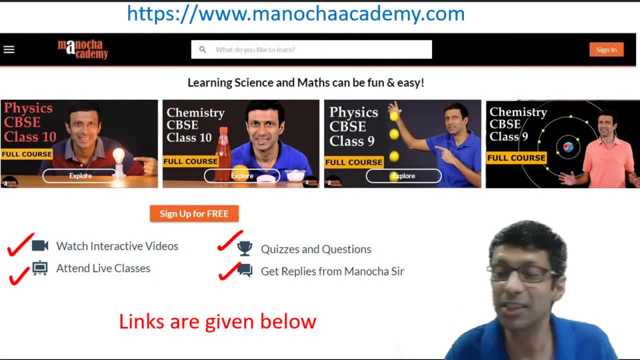 so hopefully we'll have another class on wednesday, because you know the calcutta, the weather right now is bad, but i think on wednesday we'll be having a class, a maths class, i think. so guys, do check it out. it's at 8 pm, so some of you asking where is the next live class? this wednesday at 8. 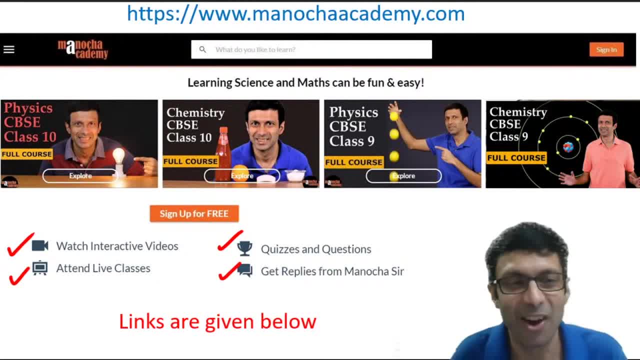 pm and i think i'll be taking a maths class on wednesday. all right guys, take care everyone. this is sandeep manocha, signing off and hope you enjoyed this class on electricity. take care, pray for your good health. i really pray for everyone's good health. 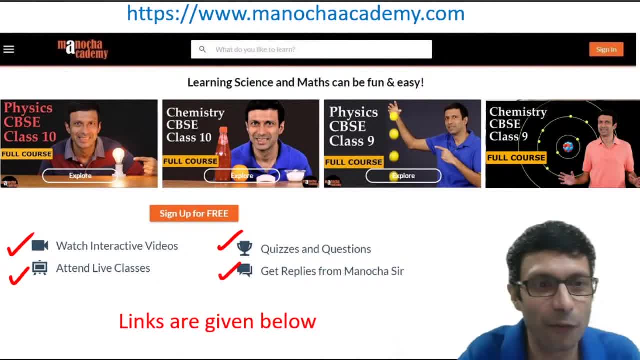 and guys, keep studying, keep learning and take care of yourself. bye.